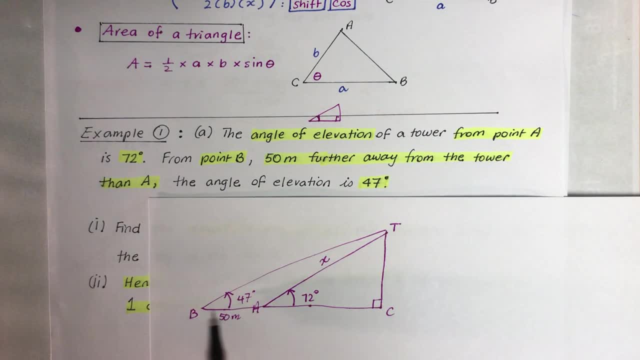 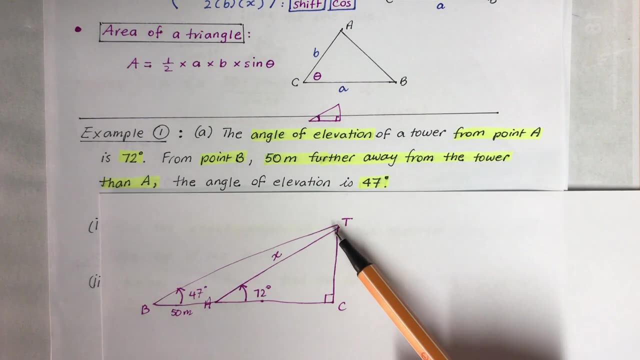 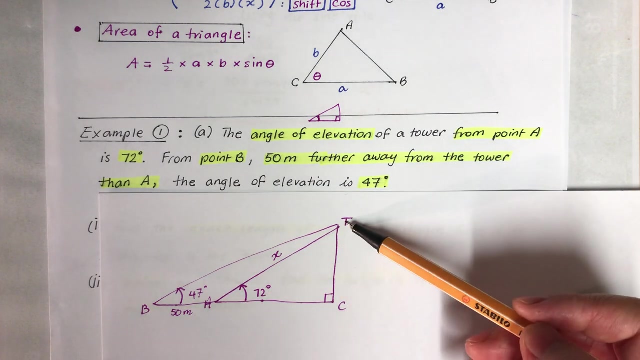 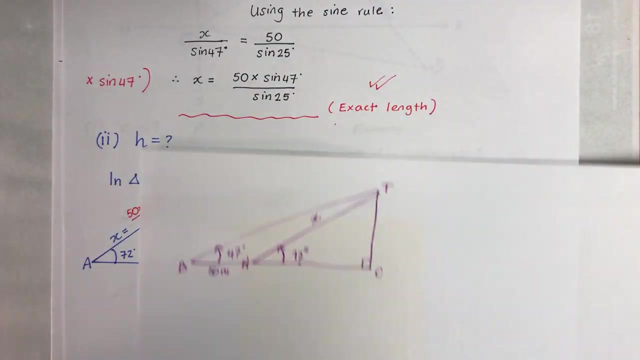 tower, okay. and then between a and B is 50 meters apart, okay. and then part a was to find exact length of 80, which is 80 here. so I'm just making 80 as an X, and now I just label the right angle triangle and then T and C so I can use that more naming. it could be easier, so I here is. 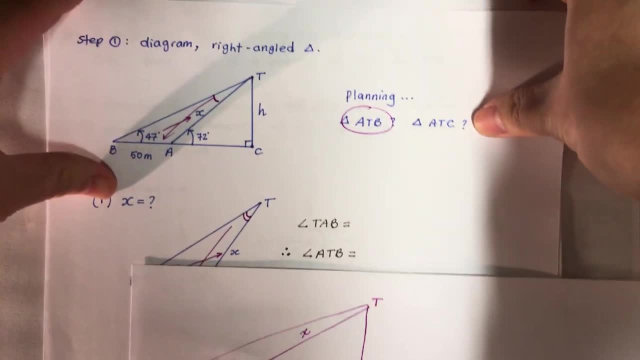 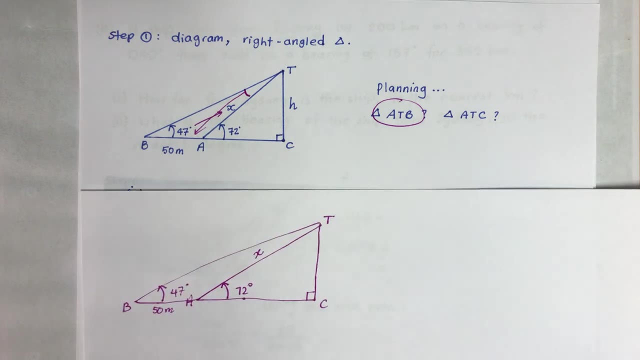 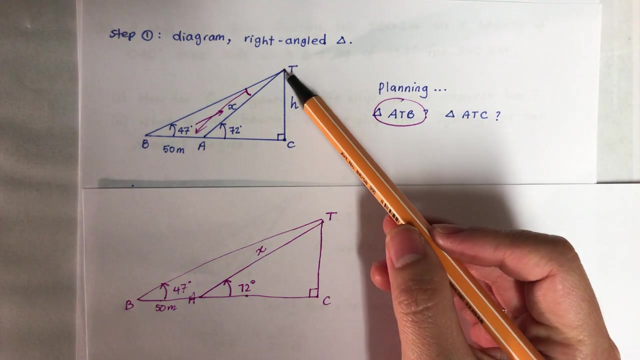 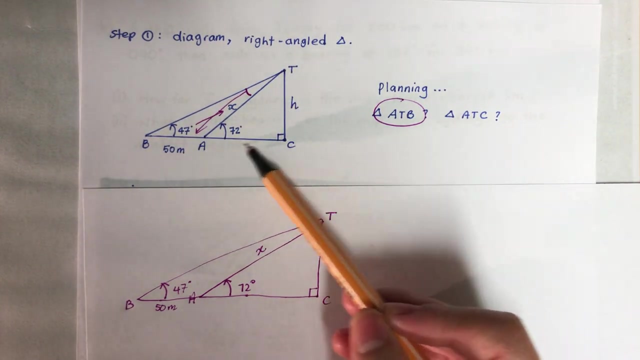 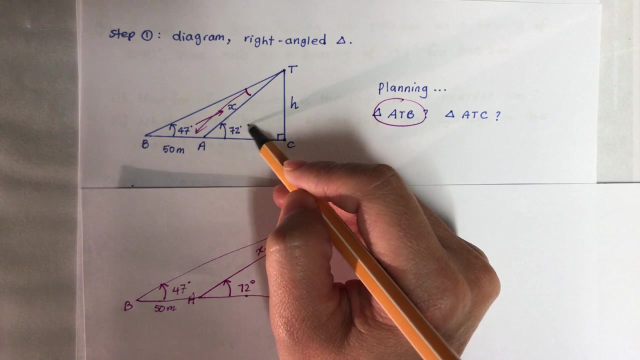 my diagram. okay, so I've done that. and then you need to think about which triangle you need to use. to X, because this AT is a common part of this triangle and this triangle, so you need to think about which one I need to use. well, this one I can't really use with that. OK, that's okay, but then I got. 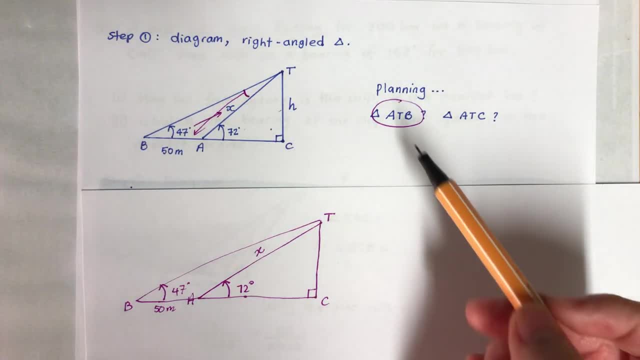 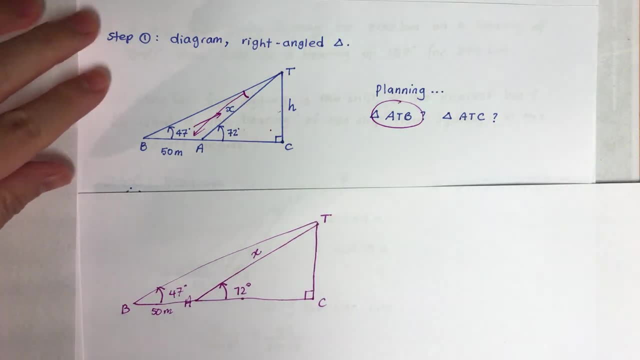 too unknown with this excited bit useless. so I'm gonna choose triangle ATB and already matched up with angle and aside. so right now we'll use ab السم side here, since we want this point narrow down goes. but then we use the angle and right angle side, this the side inside. so I'm gonna choose and triangle a TB and already matched up with angle and aside. so okay, okay. so my first triangle that I want is the. 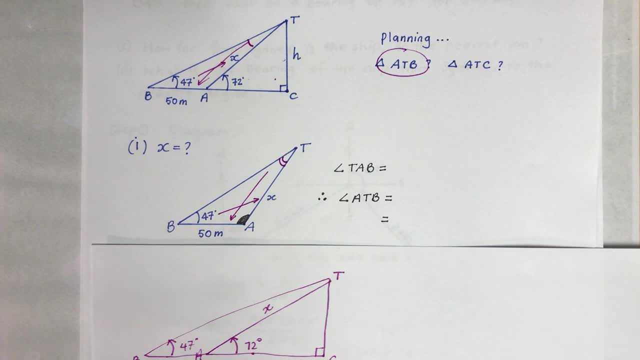 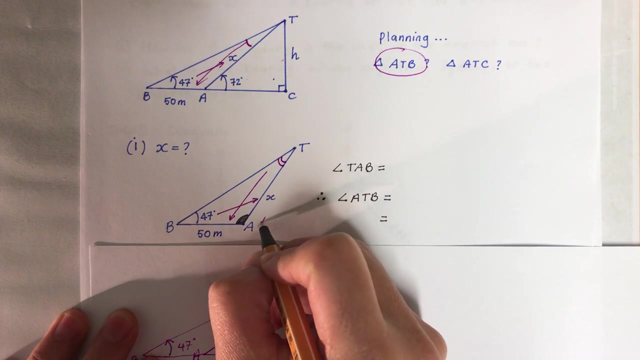 triangle and that it's. So here it is, Let's have a look. So I just resketch that And this angle I can find from here, because that's what is what? is it 180? take away 72, which is 47,, not 47,, 187 to 108.. 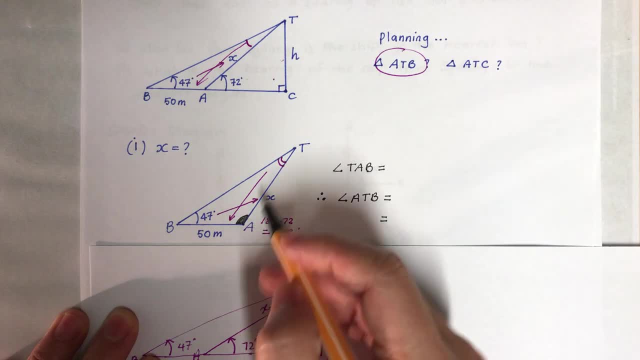 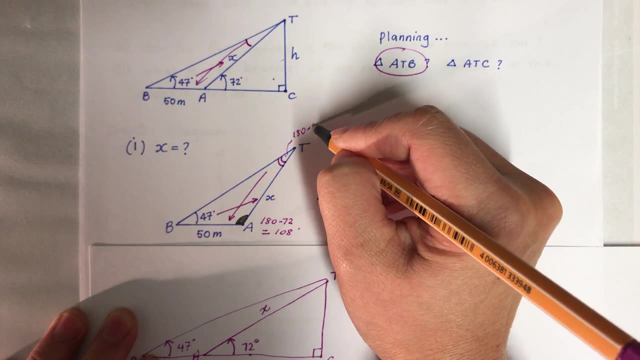 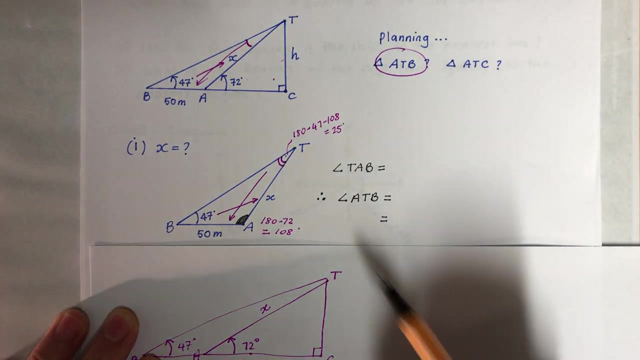 Okay, So that's my angle. And this one is easy because it's angle sum of triangle. So I'm going to go 180, take away 47, take away 108 will give me 25.. Okay, So I've got all the angles I need and the length. 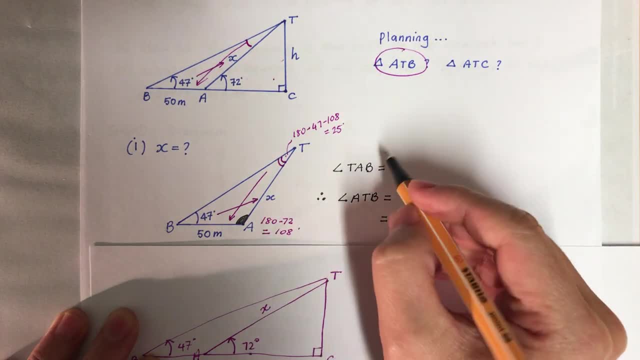 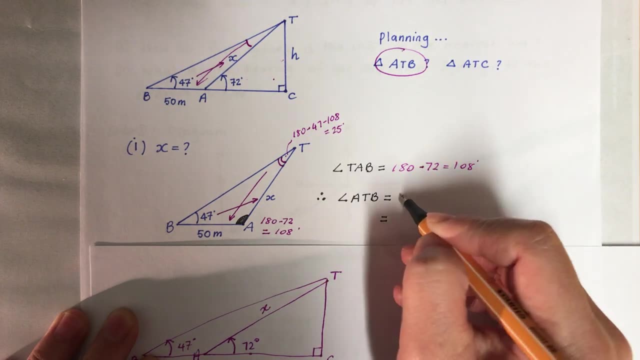 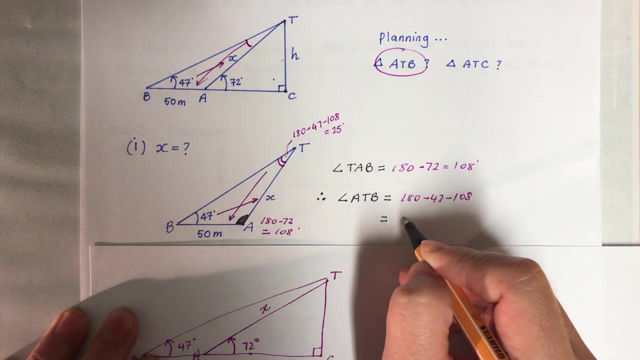 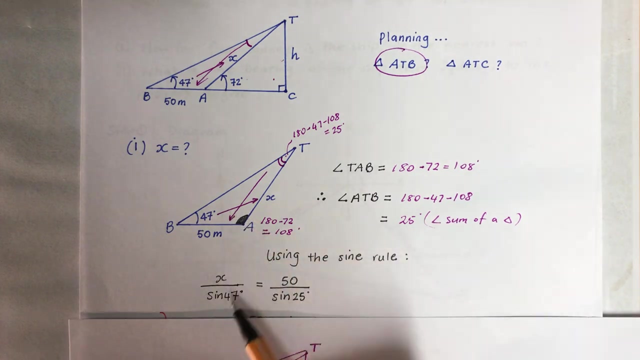 So TAB, angle TAB will be 180, take away 72. And then angle ATB will be 180, take away 47,, take away 108, which will give me 25 degrees, because angle sum of a triangle Okay. And then finally I can use sign rule. So always unknown angle or side first. So I'm going to put X and that's opposite. 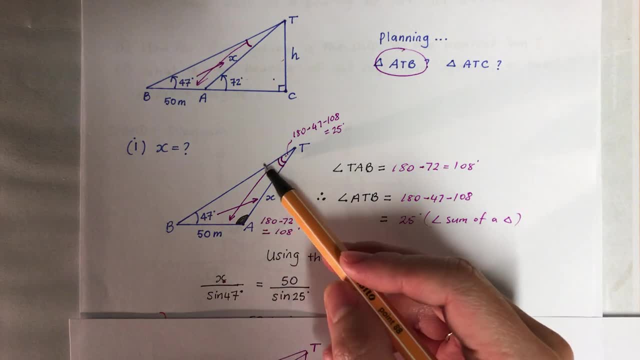 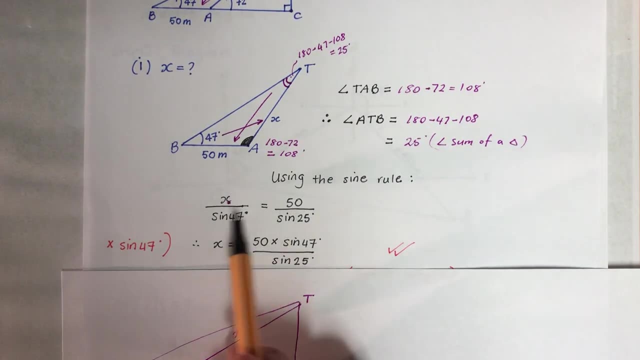 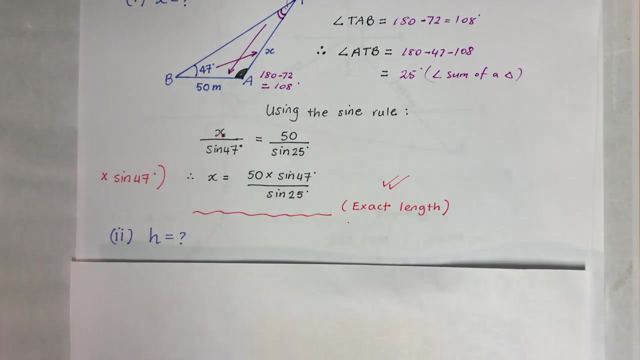 I'm already matched up. Sign 47 equals 50, sign 25.. That was 25.. And I'm timesing by sign 47, by side left with X, because I want to make X the subject and then it's exact length. So I haven't done anything. I didn't put that into the decimal. So part two was the finding a H. So I'm just going to put this diagram there, right there. 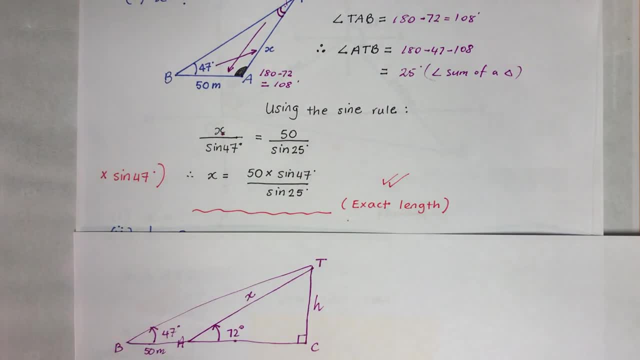 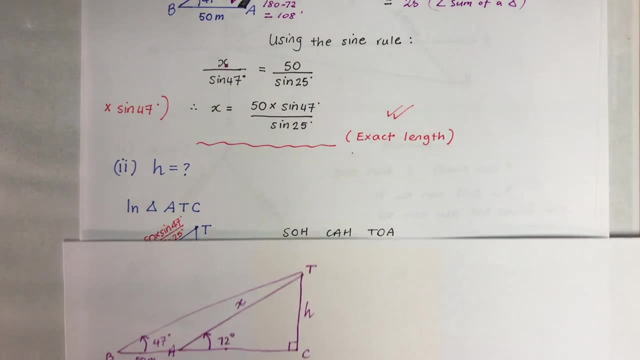 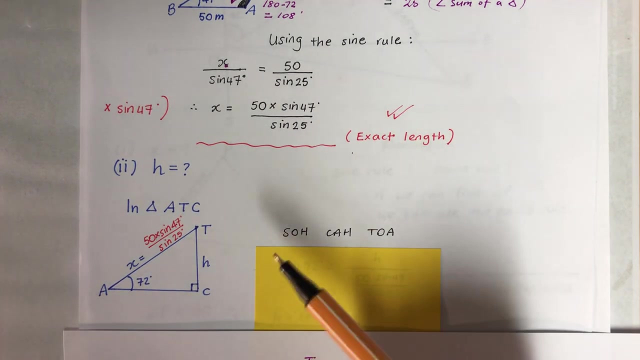 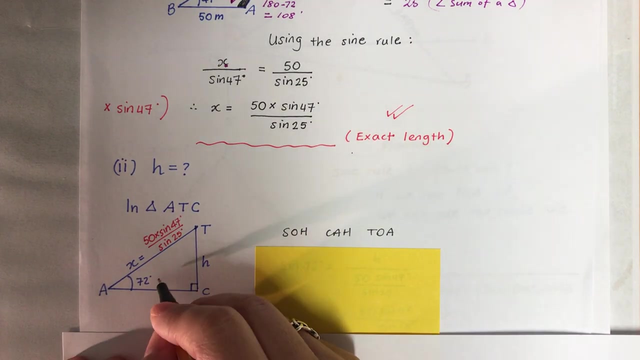 So H will be this. So obviously I'm going to use the triangle, What's that ACT? So I'll just sketch that there. And we know what X is from previous question, So I just put exact length there And then I'll have to find a H. So matching and then matching. 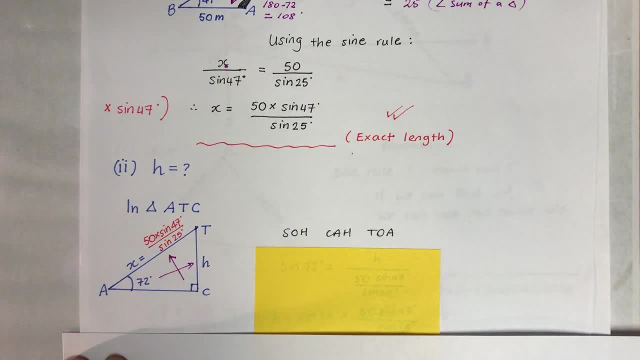 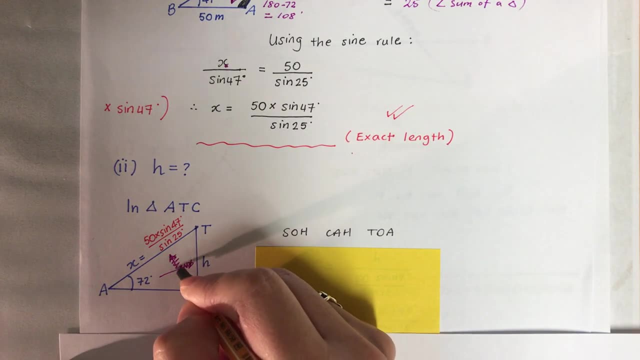 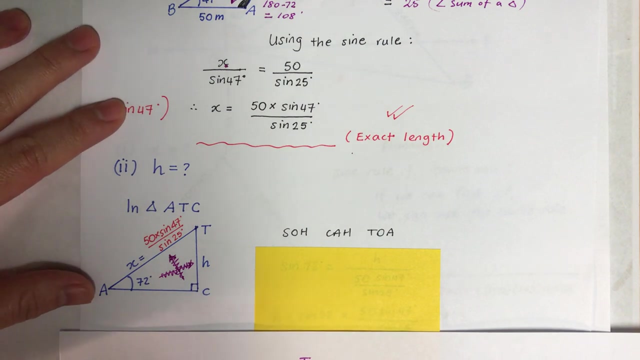 No, I don't think so. I don't need to do matching, isn't it? Because it's a right angle triangle? Yep, You need to be careful because you keep matching things. You think everything has to match, but it's not because it's a right angle triangle, Wonderful. So we don't have to do it, We just have to do it. 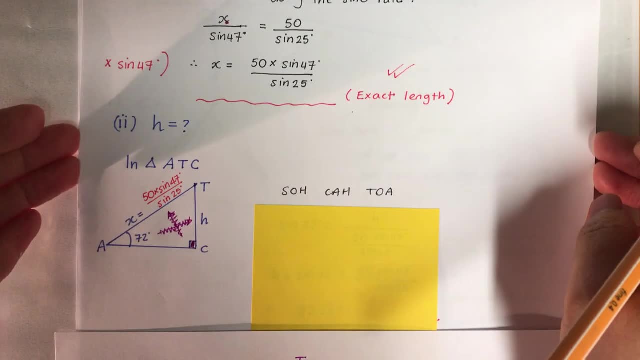 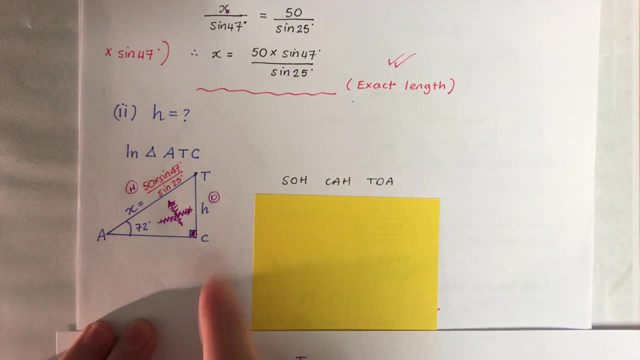 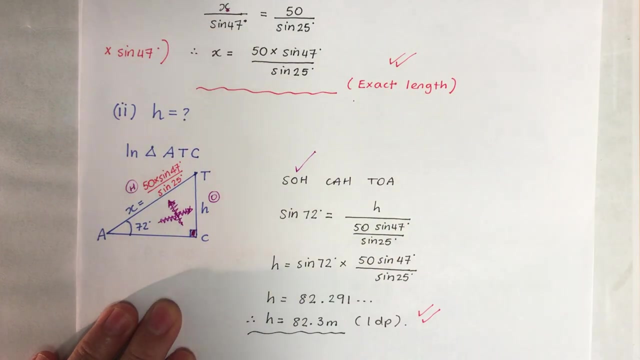 So I already written there and forgot about it. Okay, So that's my opposite. That's my hypotenuse. O and H is sine, So I'm going to do sine. 72 equals O over H, H over the exact length. 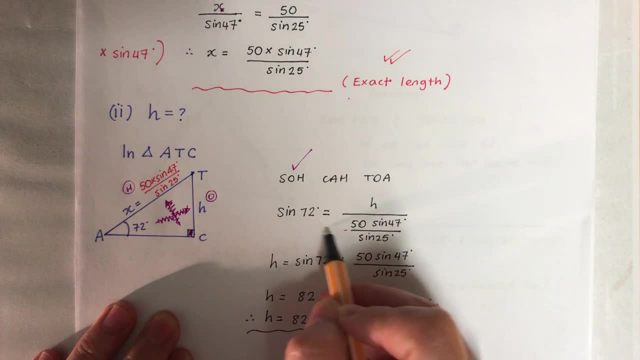 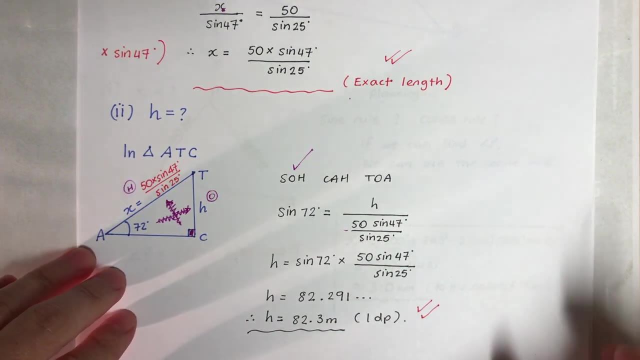 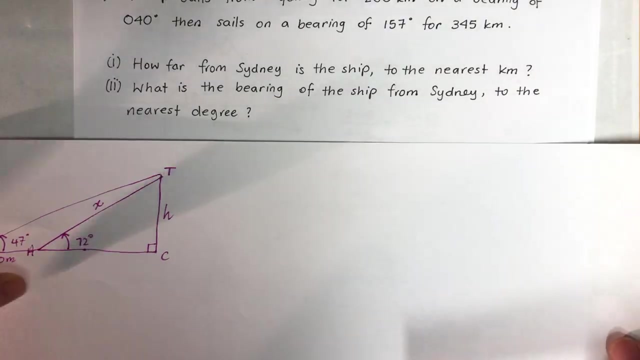 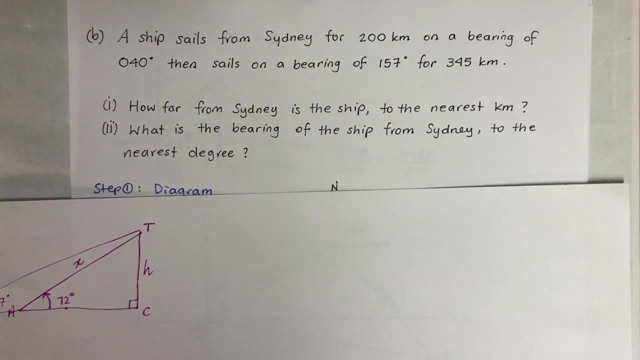 Now that means H equals times this two Yep, And then if you put that in your calculator, you will get 82.3 to the correct one decimal place. That wasn't too bad. Part B. Now I have to tell you this: It's going to be a little bit longer video, So if you need to pause it and have a break, please do so. 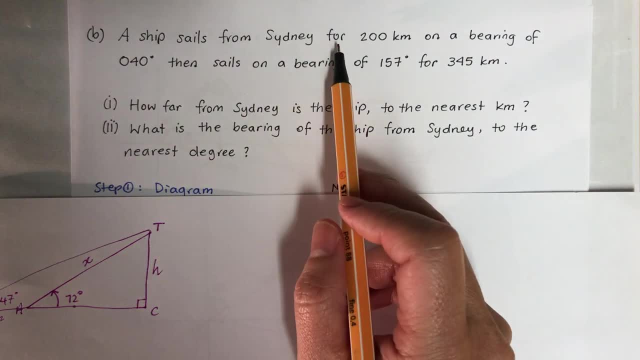 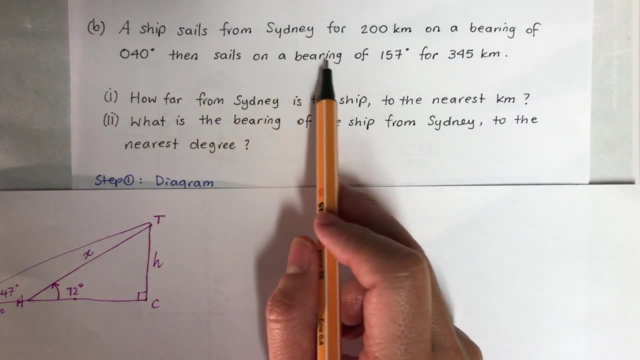 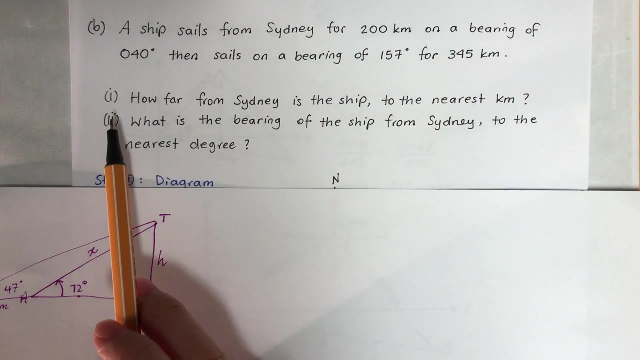 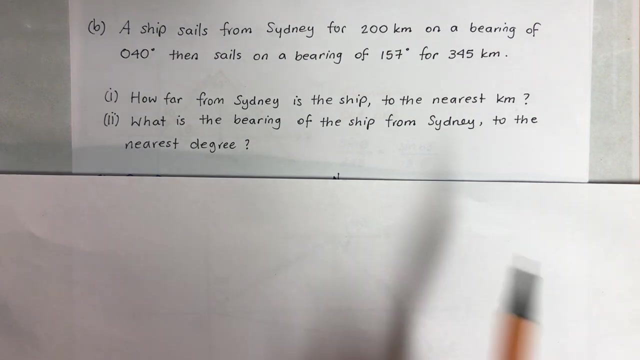 Okay, A ship sails from Sydney for 200 kilometers on a bearing of 40 degrees, then sails on a bearing of 157 degrees for 345 kilometers, And they says how far from Sydney- and I'm just going to turn this one over because I can see the other diagram- and to the nearest kilometers in a part two: what is the bearing of the ship from Sydney to the nearest degree? 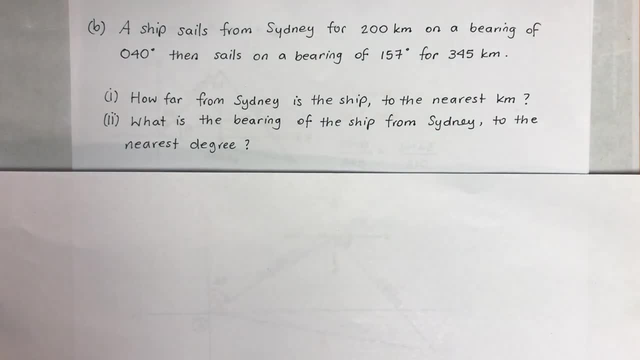 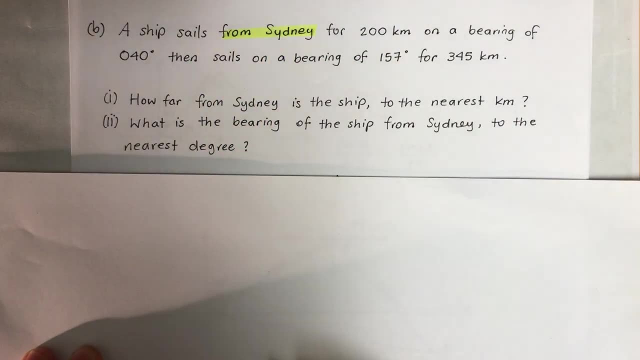 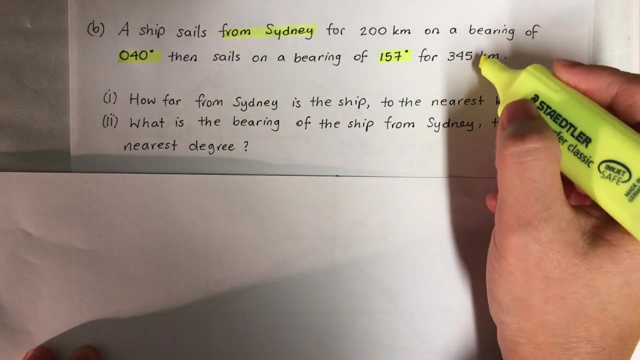 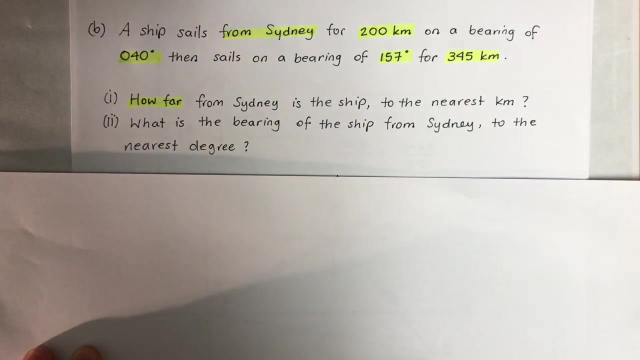 Okay, Again, I'm going to highlight this. and what is it from Sydney? That's my starting point for my bearing question. And 40 degrees and 157 and 340 kilometers, 200 kilometers, and then how far? that's a distance. and the next one is: what is the bearing from Sydney? 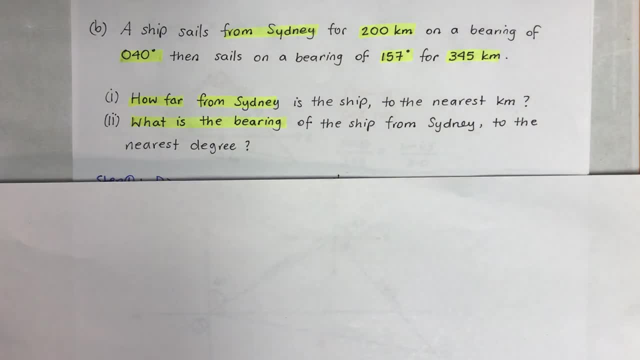 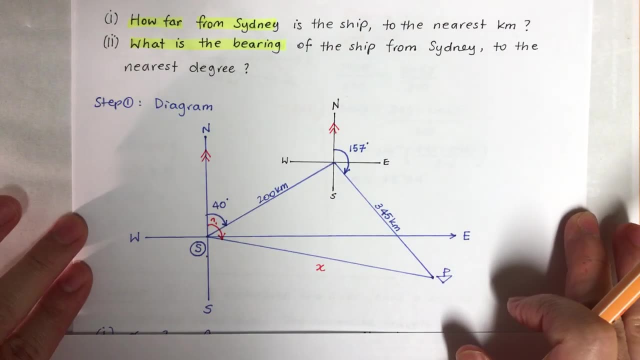 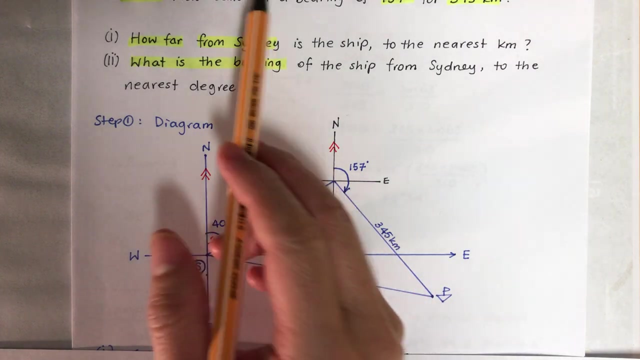 So I've done that, And first step is always the diagram. Okay, So I'm just going to show you the diagram. I've done So. all the information says So: just sketch the compass there bearing, and the first one was a Sydney was. everything was from Sydney. 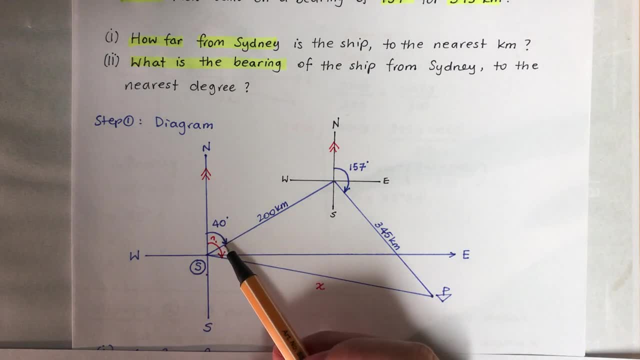 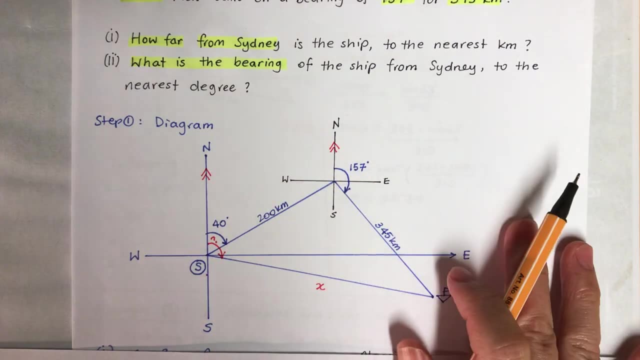 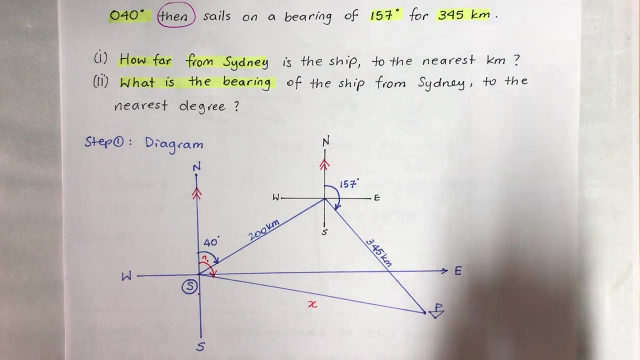 So that's my starting point. And then it was for 200 kilometers on bearing of 40 degrees. So that's a 40 degrees and 200 kilometers. And then it says: here that's the key, is saying that there's another compass. bearing is happening here. 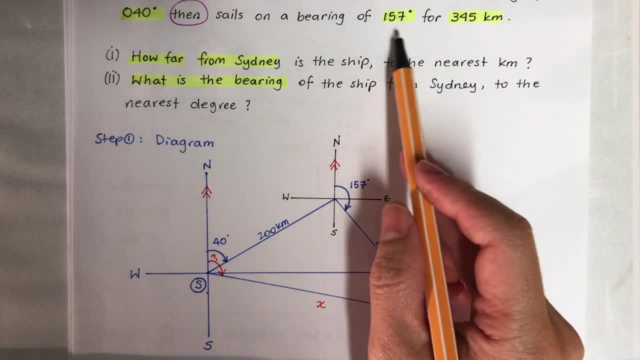 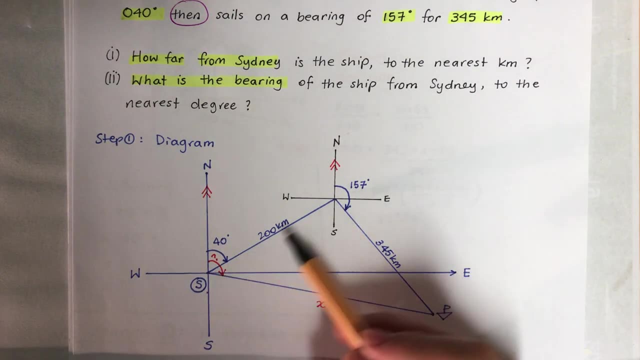 bearings were happening. so next one was 157 degrees from true north and the distance for first was 200 kilometers. second is 345 kilometers and we join them together because it says how far from Sydney to where the boat is. so that's X. I'm just gonna put X as the distance, so you need to think about this. 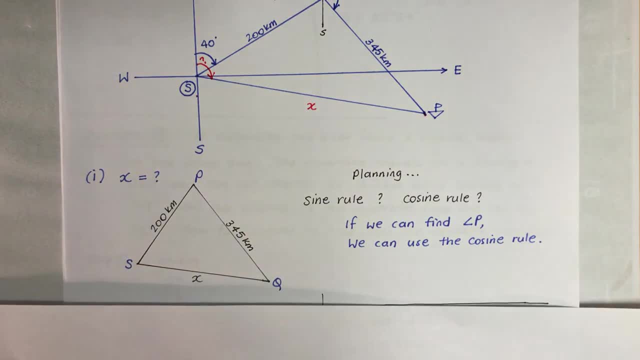 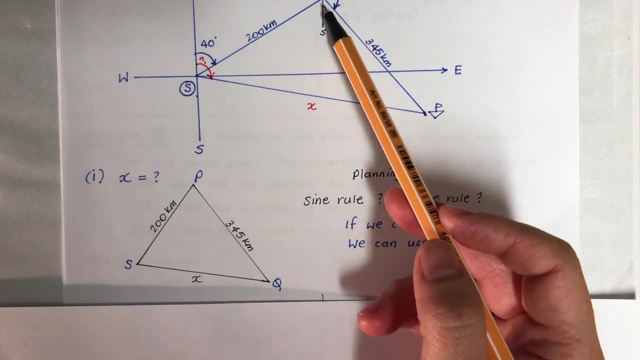 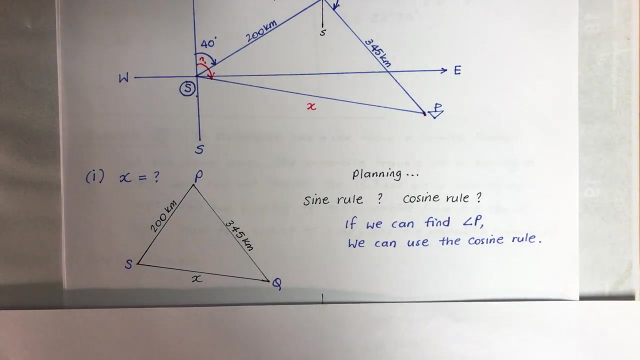 so we need to plan. so let's have a look at this. hmm, can I use sine rule or cosine rule? so I sketch this again here, so just clear up and easier for us to calculate. so I don't, I don't know, I don't know. think we can use sine rule here because I can't really match up with any angles. 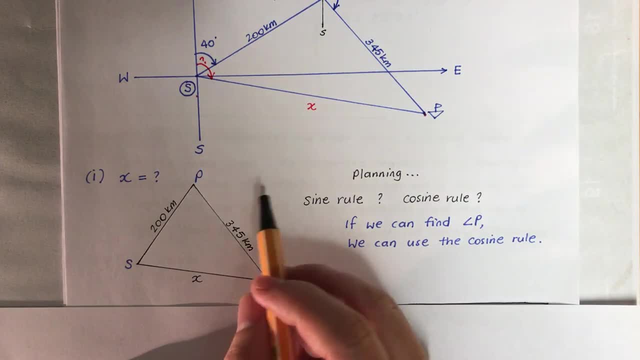 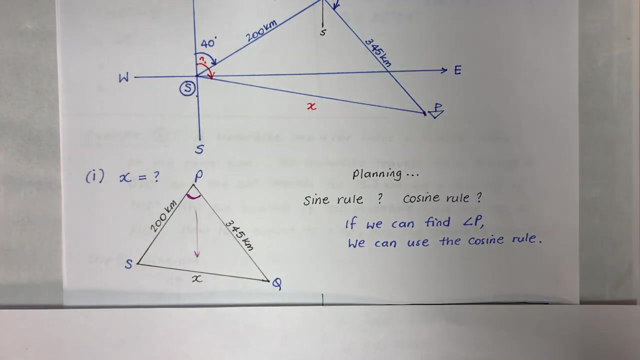 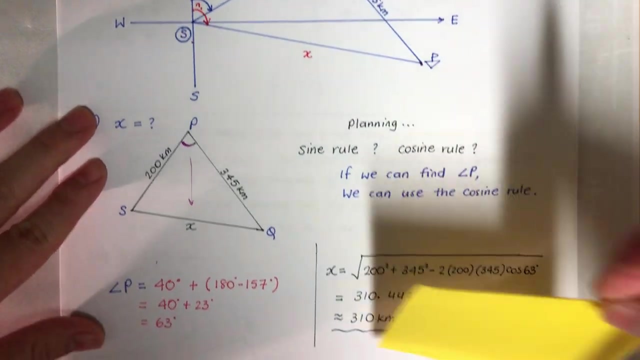 I can't see any angles there, but if I can find the angle P, I can use sine cosine rule for this one, because, remember, cosine rules, you need to have all this side covering, almost like protecting the angle, and then we can do. that might just cover this one up, эта keima. 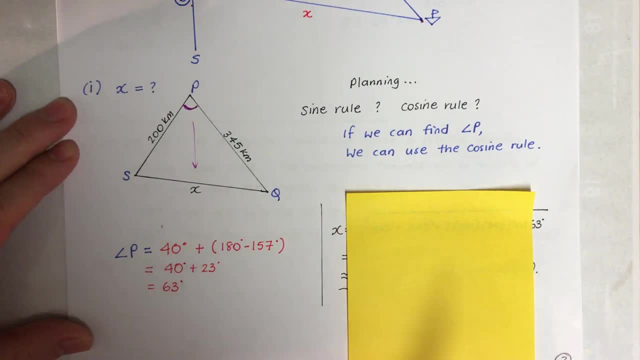 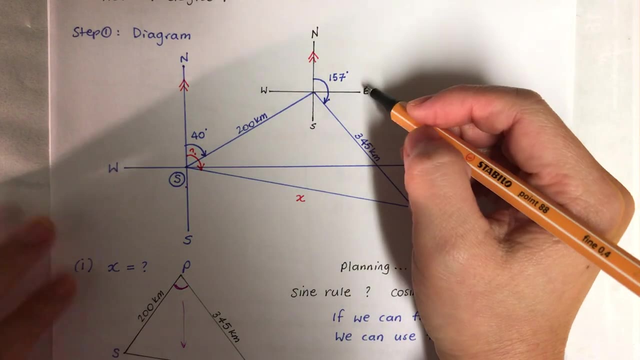 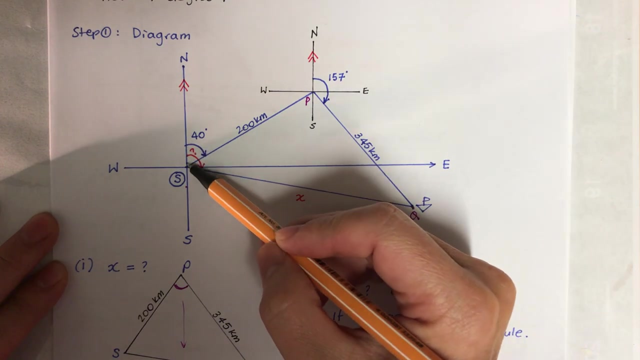 so find the P. how are you going to find the P? it'll be. I'll have to go up repeat. I'll just name the P here. thank you, so P will be now. can you see that's looking good moments. there is a help with numericias. 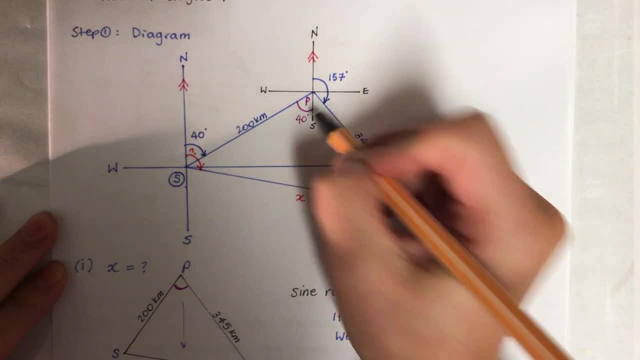 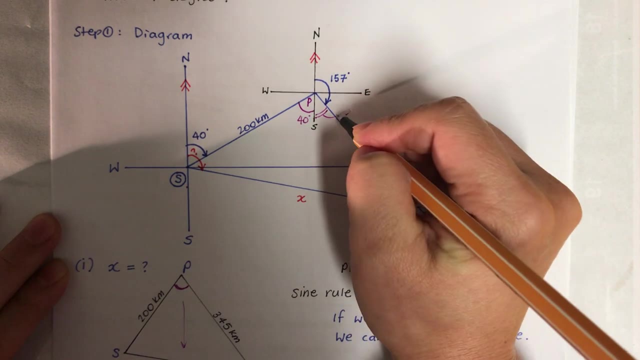 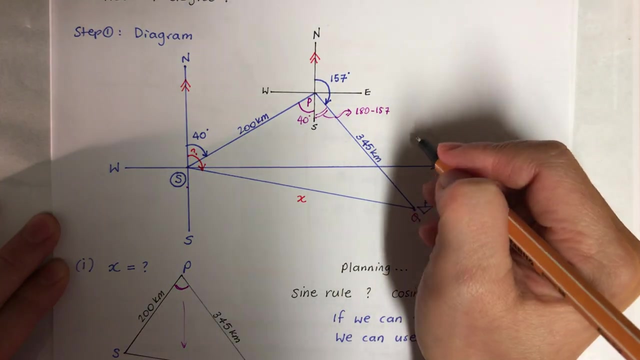 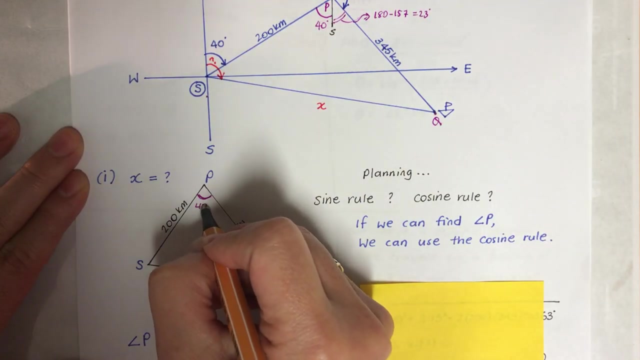 if it just isn't it still there. yeah, that looks good. yep, so that's good. and here is what: 180 take away 157. yeah, so what's that going to be? it's 23. so what's the p going to be? it'll be 40 plus 23 will be 63. 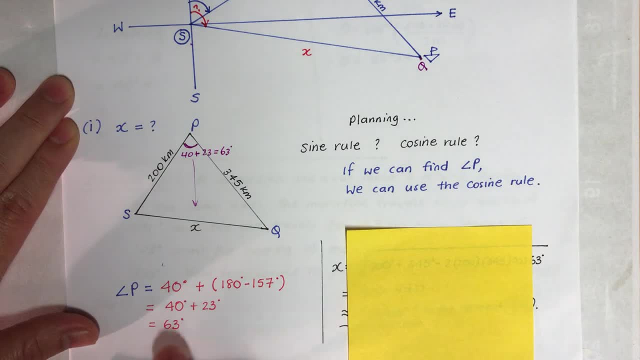 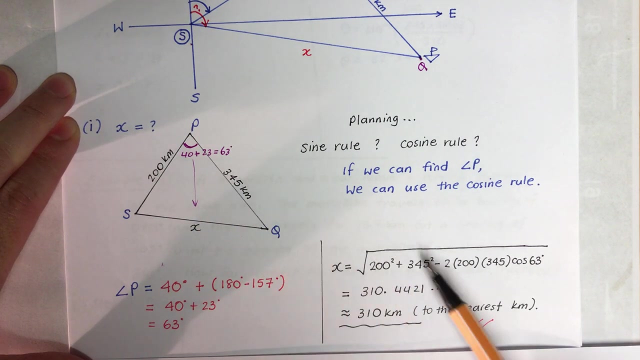 voila, there you go. so we got 63 right there. so now we have to use- i'm going to use the quicker version of the finding x using cosine rule, so it'll be 200 square plus 345 square minus two times that. times that and the cos 63, where it's the opposite to the side, and then, if you, 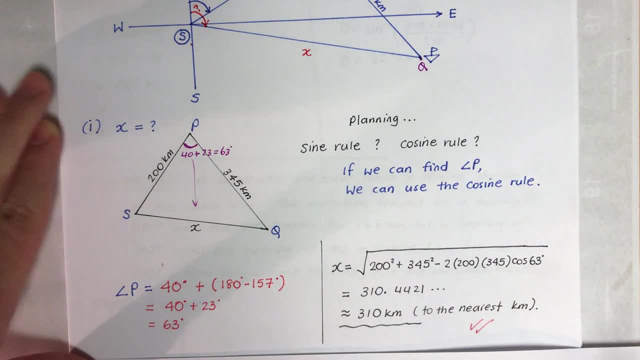 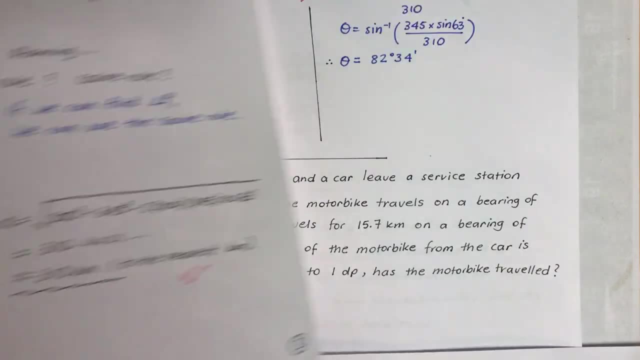 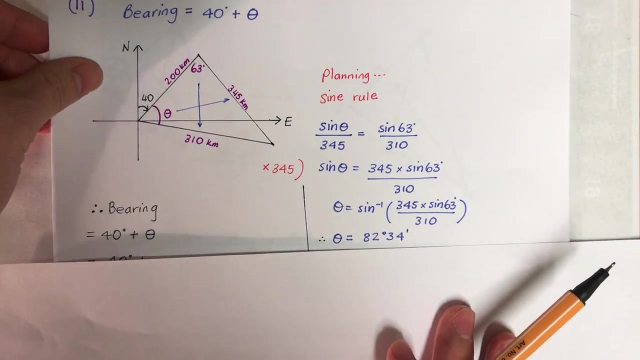 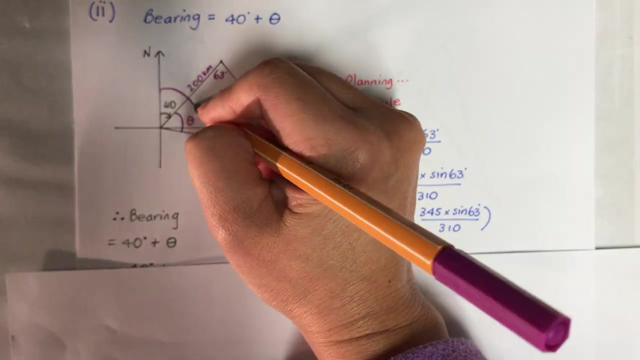 put that all that in your calculator: to the nearest kilometers will be 300 and 10. that's just finding the part one. how far the distance? now part two: we have to find the bearings. so that'll be this part. this is the bearing, isn't it? that's what we have to find, the bearing. okay, so that means. 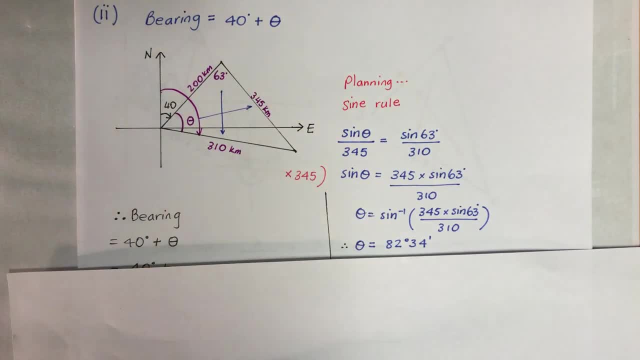 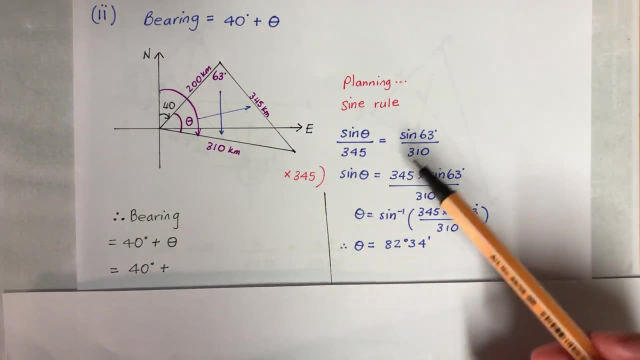 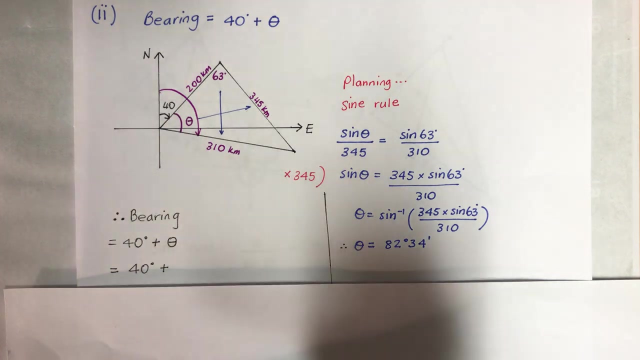 40 degrees, the theta part will be the out bearing okay. so again, we need to have a bit of a plan. so we need to think about if i could just match up with these and these, that'd be fantastic so i can find the theta okay, because we need to find the theta to. 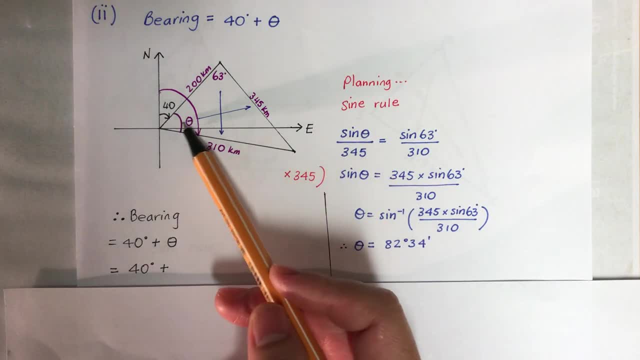 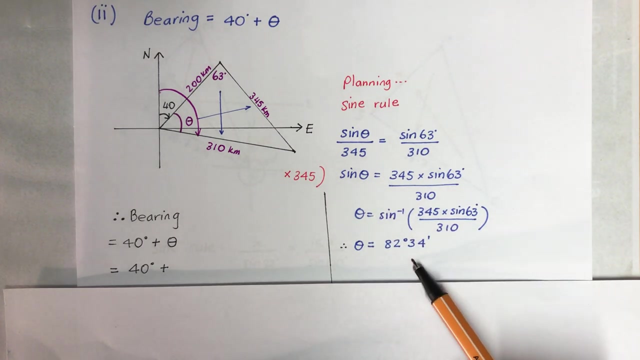 find the whole bearing. so let's do that: sine theta over 345 equals sine 63 over 310 calculation. just remember it's angle. so you've got to do a shift sign. but that's not the bearing, is it? that's just part of bearing. so whole bearing will be 40 plus theta, which is 82 degrees and 34 minutes. and if we do that, 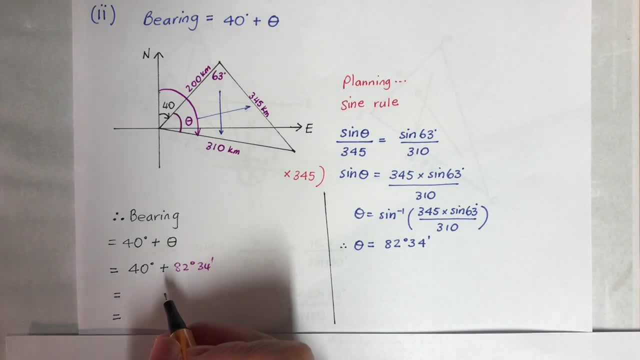 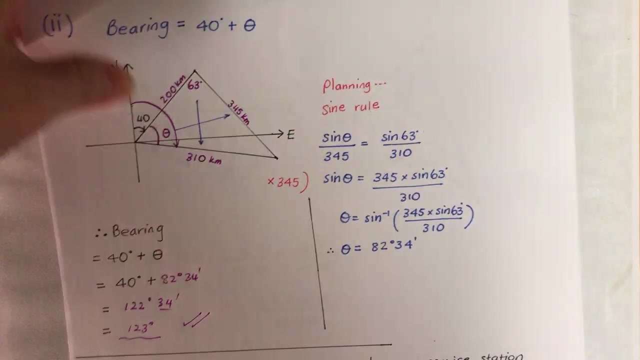 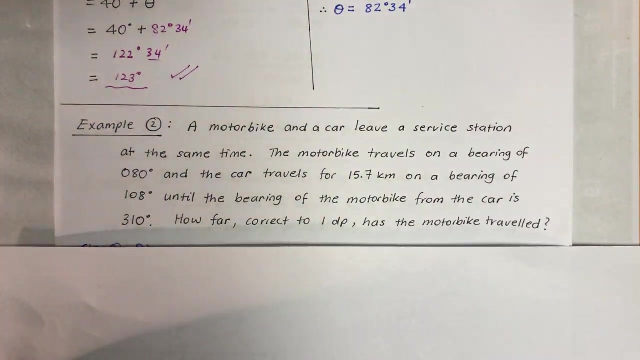 what do we get? a hundred and 22, 34 and, to the nearest degree, 123, because it's more than half. okay, so that's good done, excellent part. example two now. a motorbike and a car leave a service station at the same time. the motorbike travels on a bearing of 80 degrees. okay, so I'm going to. just as I read, this is: 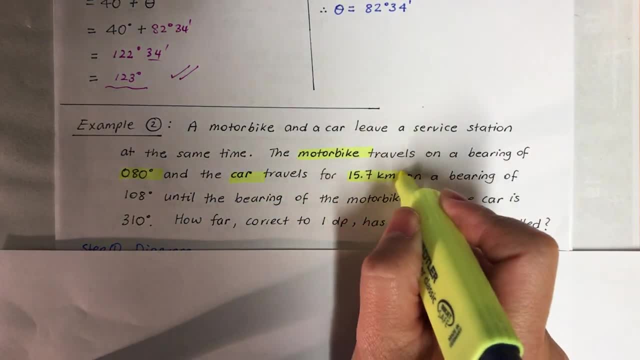 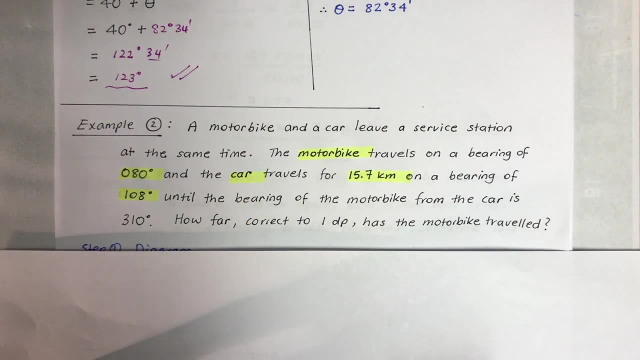 highlighted, and the car is a 15.7 kilometers and bearing of 108 until now. this is going to be a little bit tricky until the bearing of the motorbike from the car is 310. so key word is from the car. it's not from this service station, it's from the car. and how far correct to one. 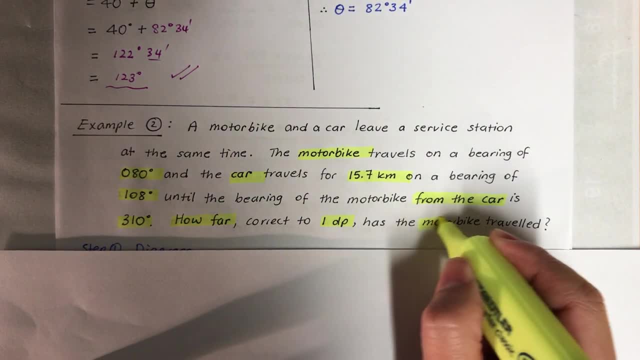 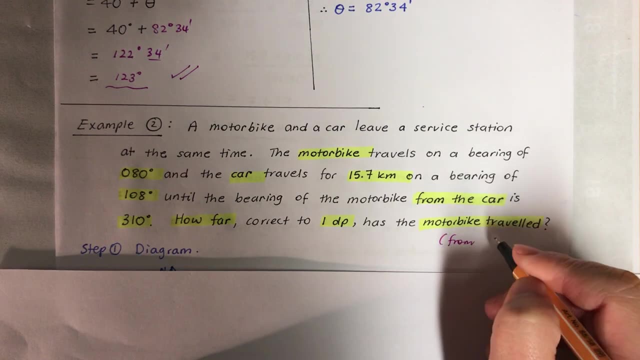 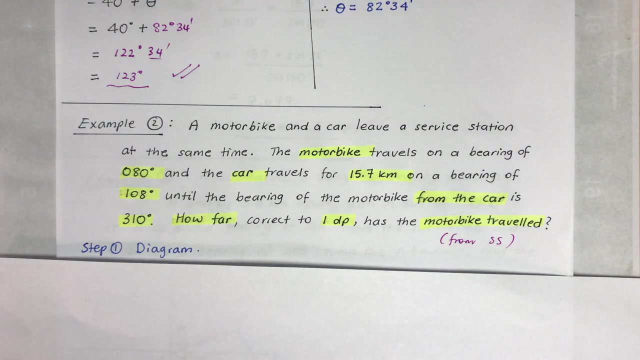 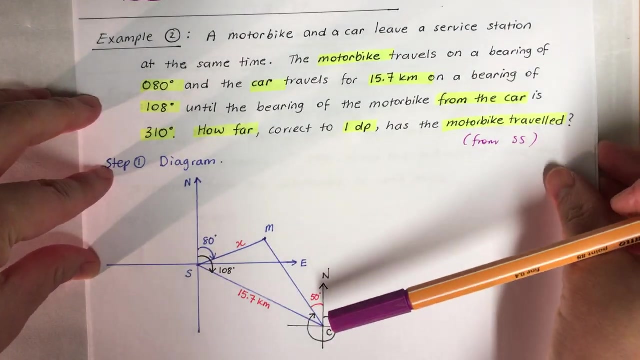 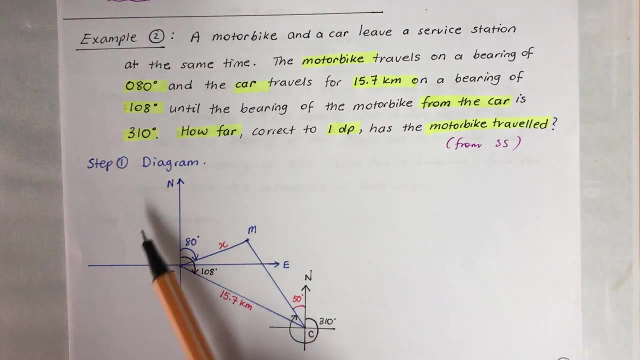 decimal place, has the motorbike traveled? now, I think here, key word is from service station. okay, from service station. so we need to think about that. okay, of course, important thing before we start anything else: step one is the diagram. so this is the diagram already prepared for you. it's like a cooking show, isn't it so? 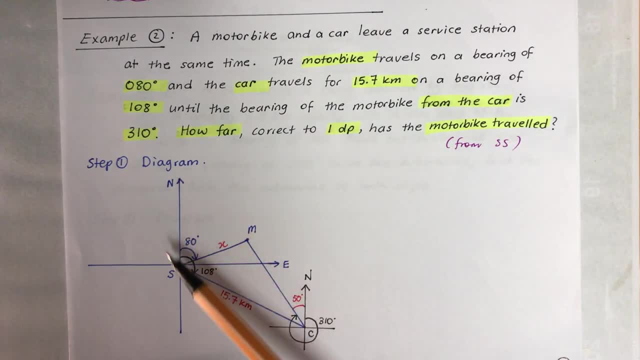 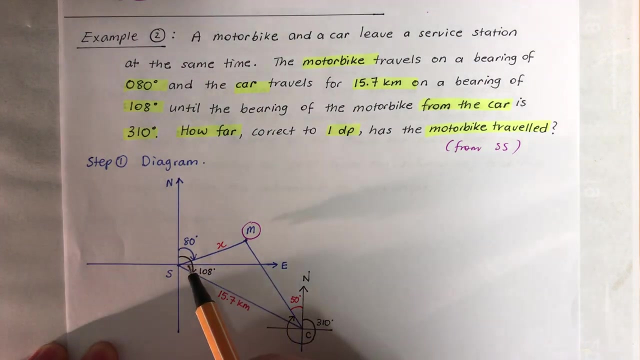 diagram is here and north, and then that's a service station and both of them started together, so the M for motorbike and the C for car. so bearing and bearing is around 185 degrees and, and, as you see, 296 degrees, the M for motorbike. 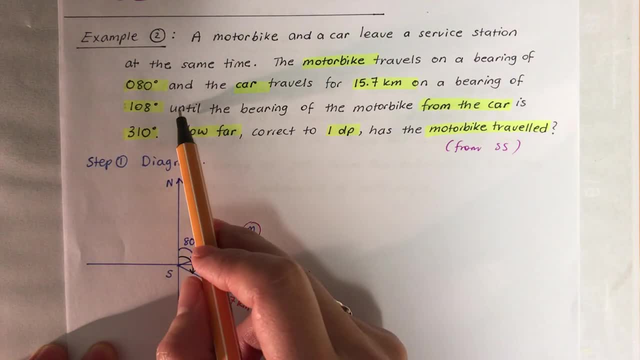 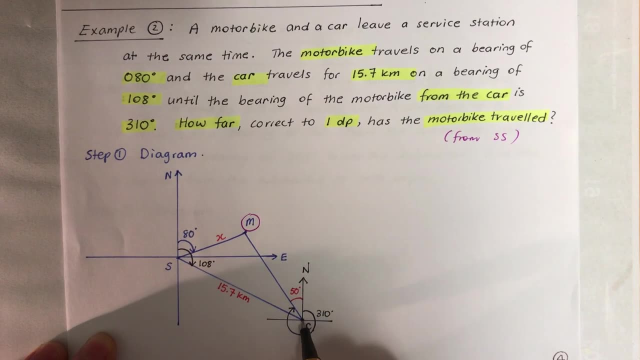 is around 880 degrees for motorbike and the but 108. yes, so the car was 108, so they're separated and the distance was only given for the car, and this is the part you have to be very careful now- from the car. so the your starting point has changed now it's not the one from the car, so it's a specific given to the car from now. so you have an option for one car if you are stood on some of the other하� and- and this comes from the Horror association, something like this- it's a very common 思. 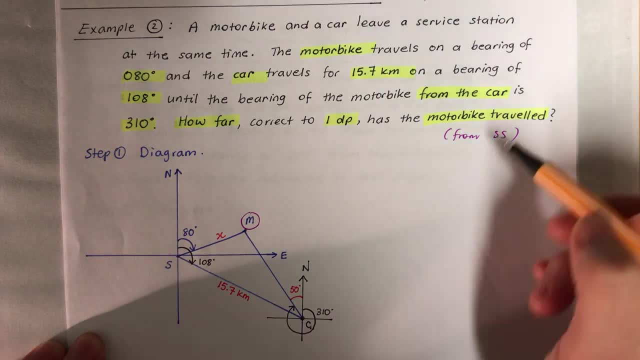 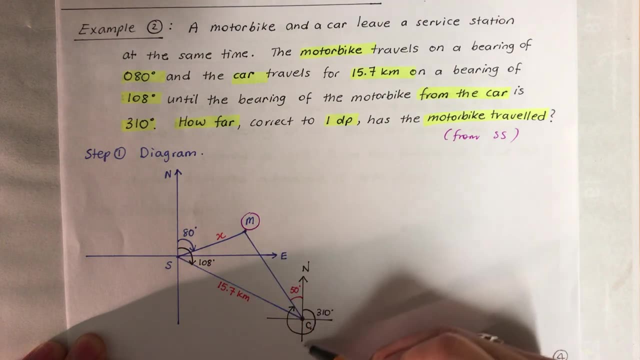 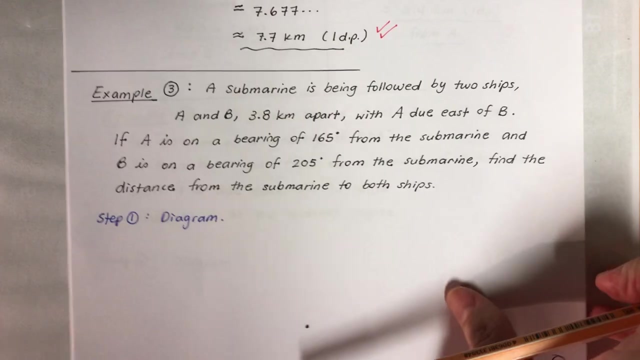 station anymore. it's the car and it's 310 motorbike. where the motorbike is is the 310. okay, I just put the 50 degrees so that you know it's a 360. that little part is 50 degrees. so as long as you could actually sketch that, that is very good, and I'm just gonna continue with this. 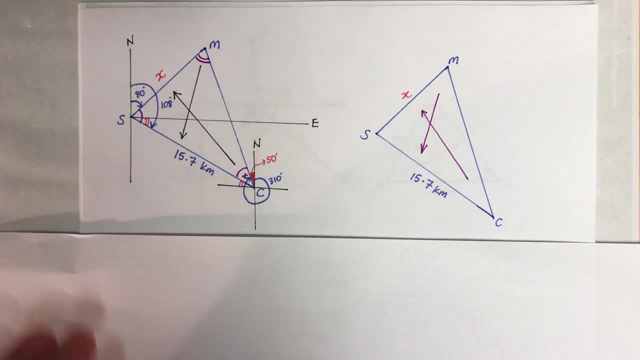 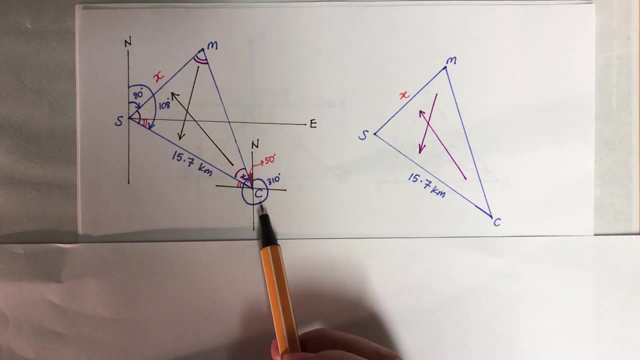 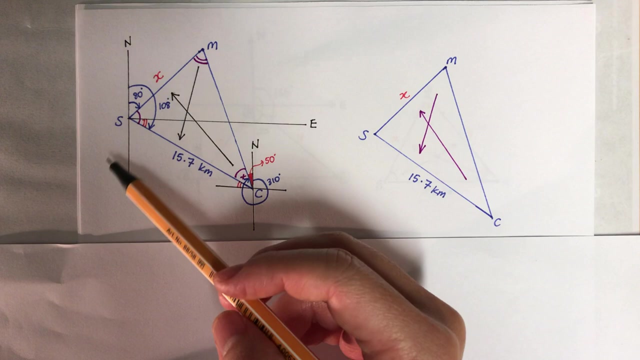 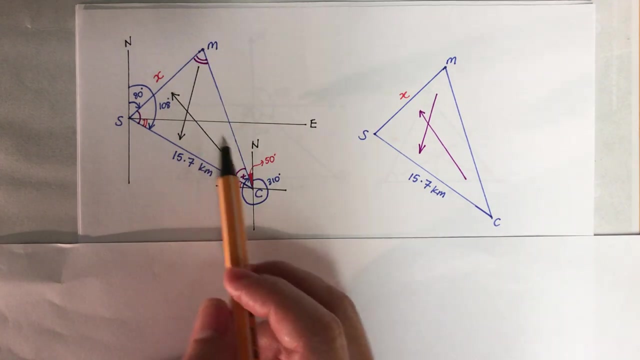 so I sketched a little bit further and put all the information I want to use. so that was a 50 degrees now to find this distance, how far, so half, is the motorbike traveled from the station. so that's this what it is and I sort of trying to match up. remember trying to use a sign rule if 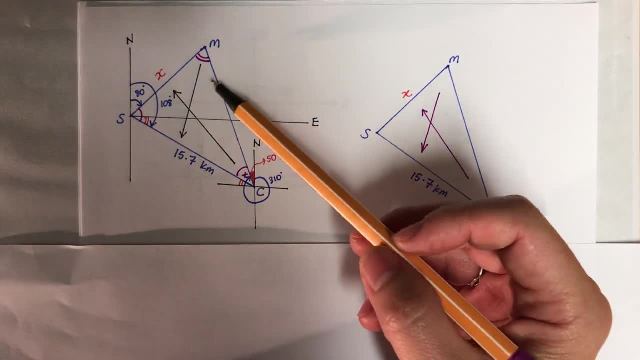 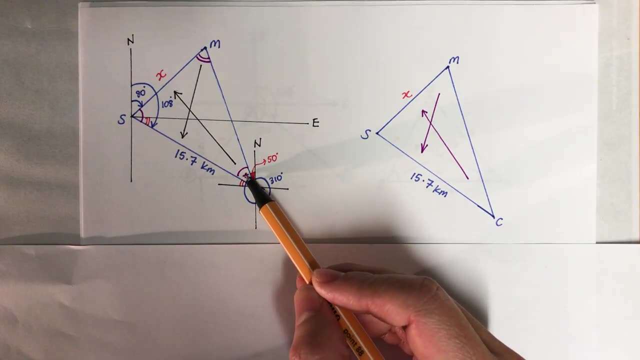 you could have to match up the distance. but you could have to match up the distance. so I'm just, if you kind of, obviously you use a sign, cosign row, but if it's a sign, so I'm just trying to match up and it does work if I can find this angle and I think I 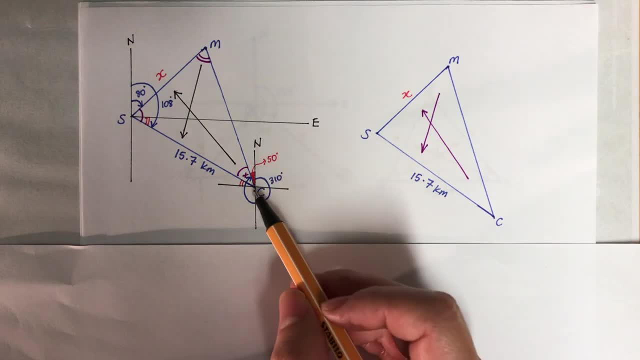 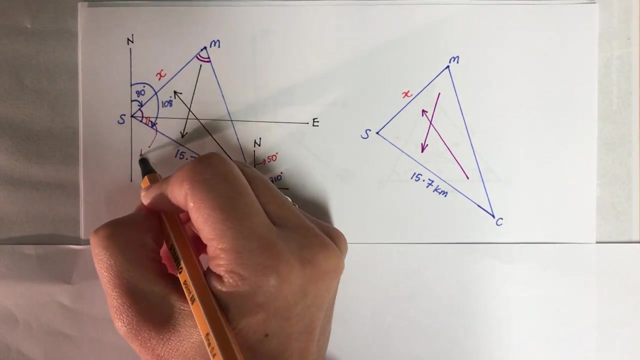 can work around it because there's a lot of bearings here, so I can sort of work it out. so that's 50, and if that's that's like alternate, isn't it alternate? so how do I get this angle? it's hundred and eight. take away 90, isn't it? because 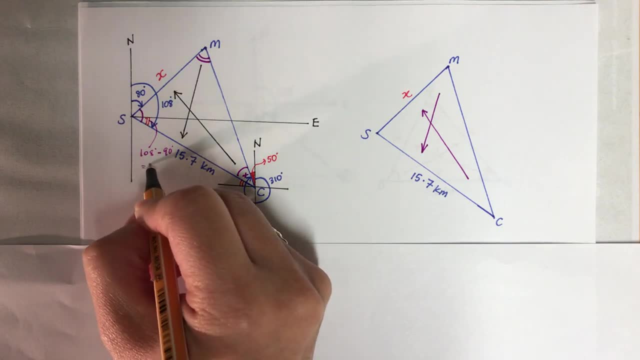 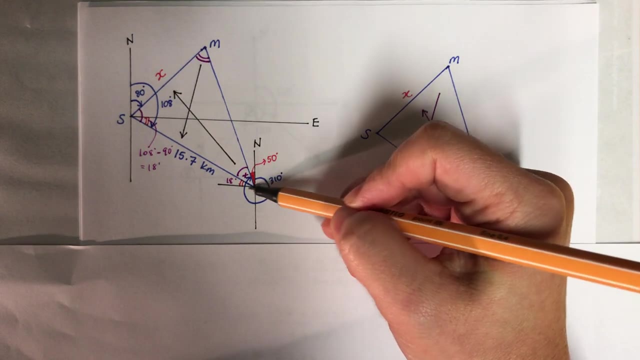 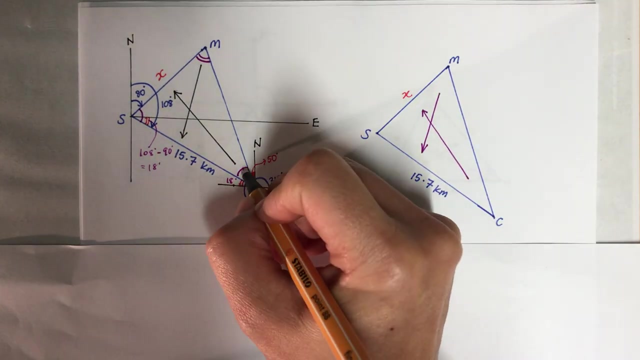 hundred eight, take one ninety, I will get 18 degrees. okay, so that for that little part is 18 degrees, now whole thing is 90. so if I can get 90, take away 50, takeuper 18, right, I will get this angle. so this angle was night. 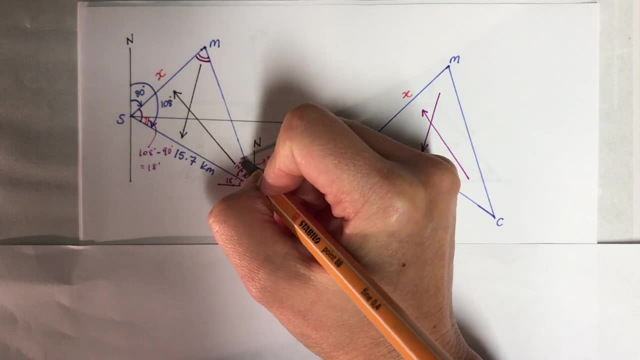 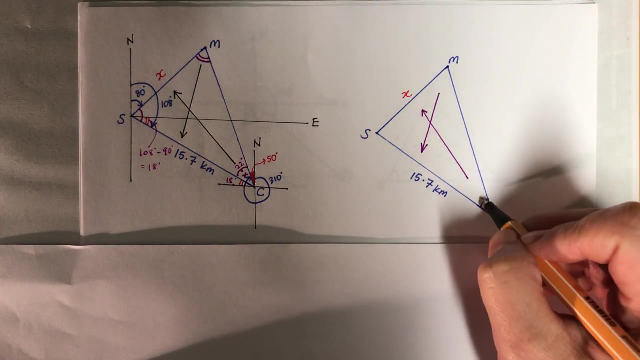 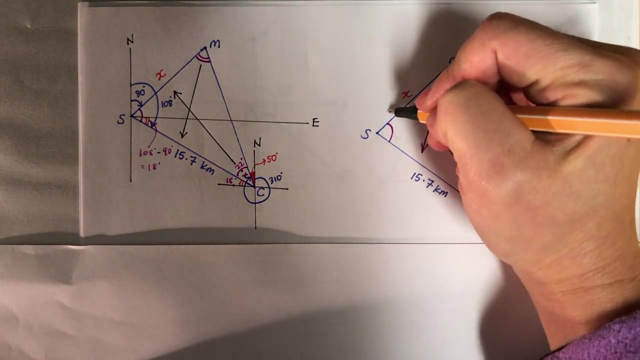 take away 18, take way 50, It'll be 22 degrees. Yeah, right there. So I'm going to put 22 here. And what was this one? And this one is easy, actually, It's what? 108 degrees. take away 80 degrees, which is 28.. 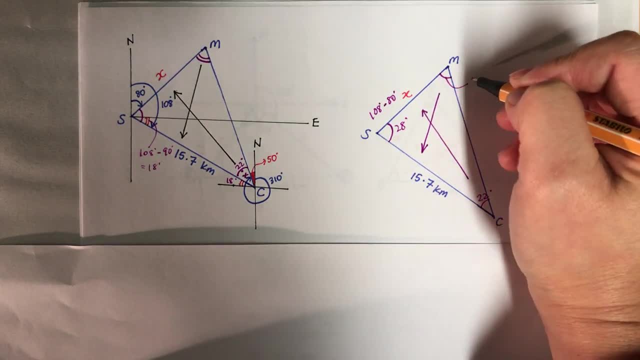 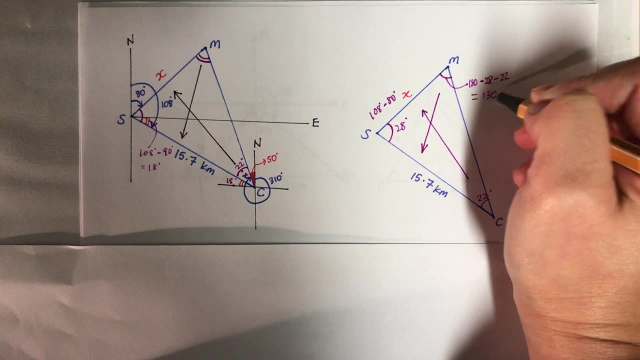 Okay, And the angle, sum or triangle. I can find this one: 180, take away 28,, take away 22,, I'll get 130.. So that's 130.. Okay, I think I've got everything I need. 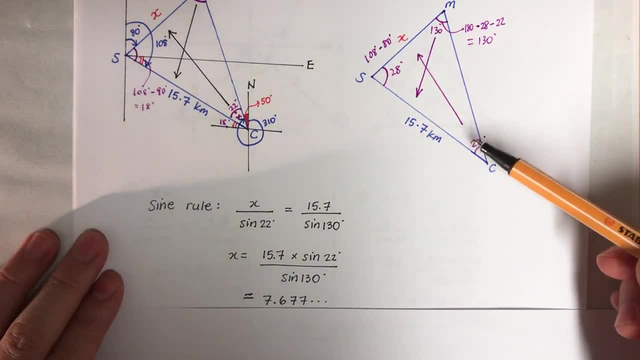 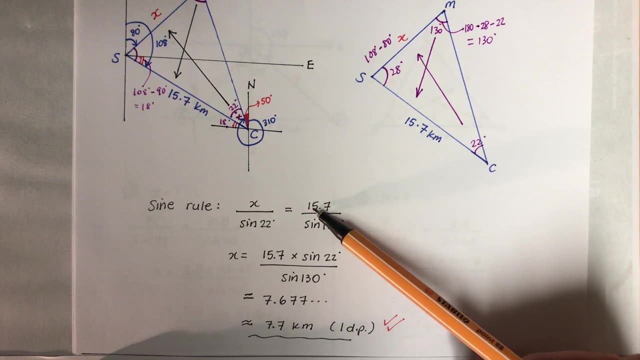 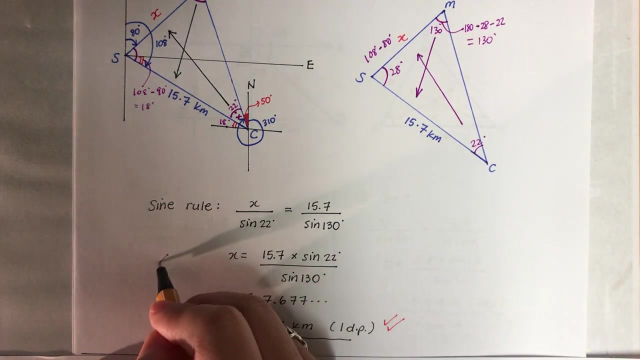 So to find x, I will go using sine rule. So I'll go x over sine 22, and then 15.7 over sine 130.. And I timespeed, I timespeed sine 22 degrees on both sides. 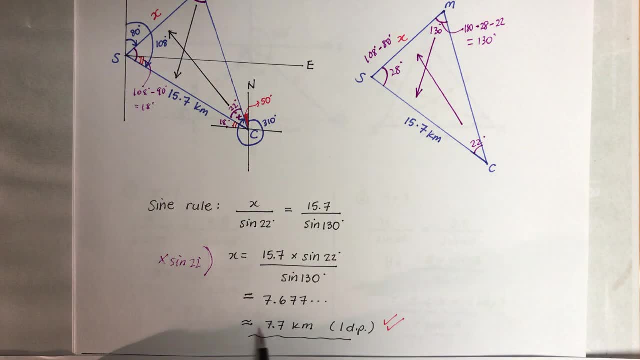 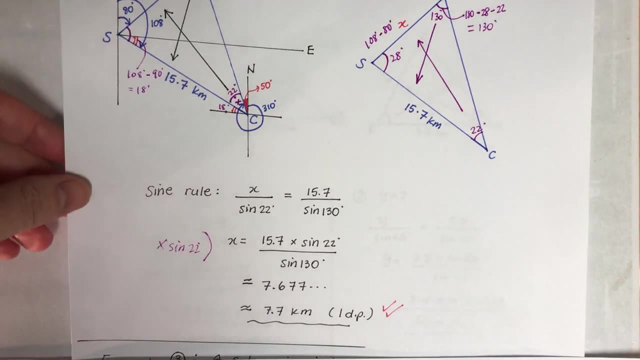 And I'll make x the subject: Da-da-da-da-da. 7.7 kilometers, one decimal point. Okay, Excellent. Now did I tell you this is going to be a long one, So just pause it, have a break, come back. 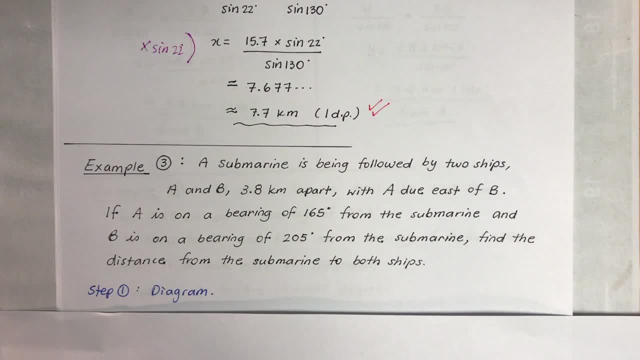 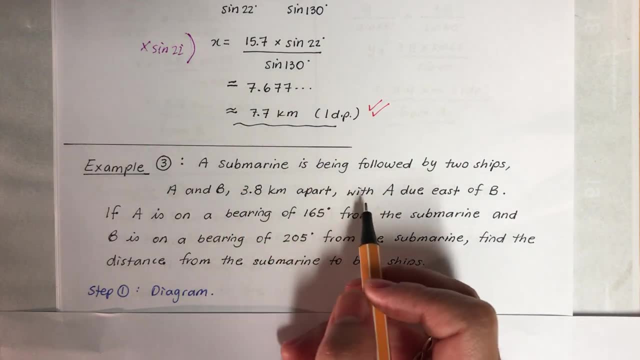 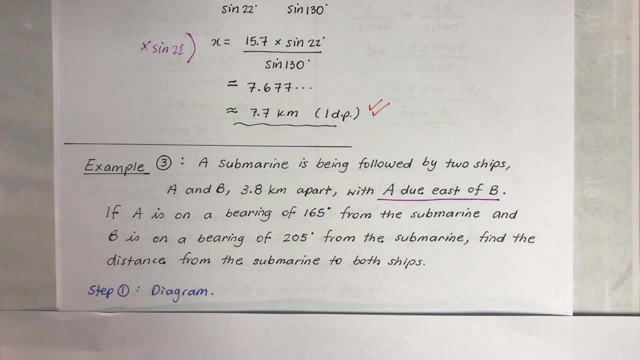 Okay, So next one Summary is being followed by two chips, A and B, and 3.8 kilometers apart, with A due east of B. Okay, So that's something you have to be careful about If A is on a bearing of 165, so again, I'm going to put that one in there. 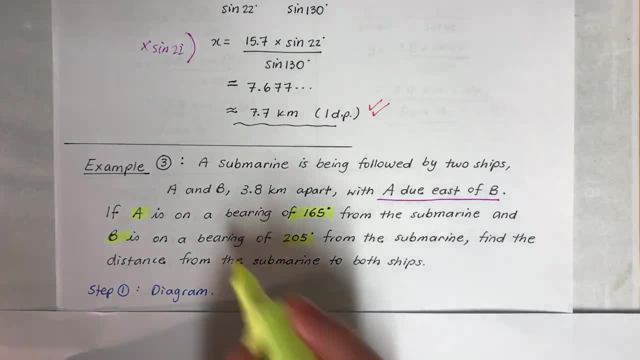 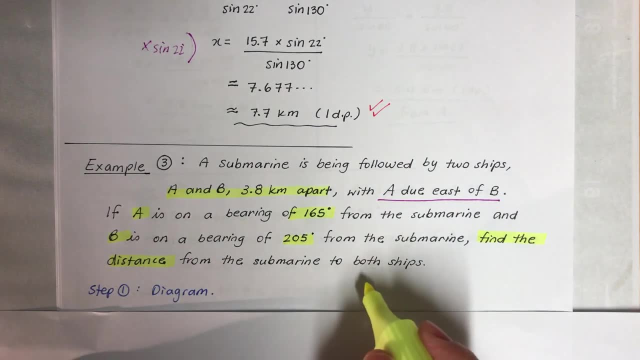 And then B is a 205.. I'm going to put that one apart. Find the distance from the submarine to B. Both chips A and B. So find that Okay. So diagram It's not too bad. Just think about the diagram. 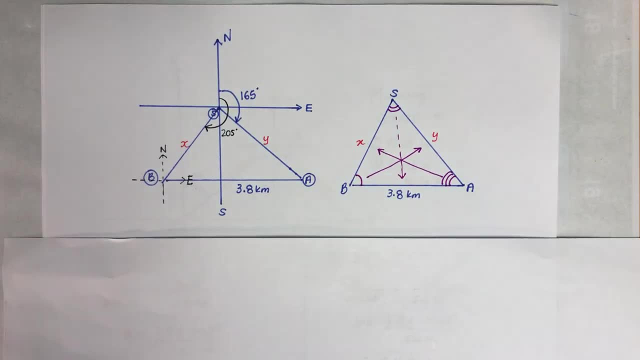 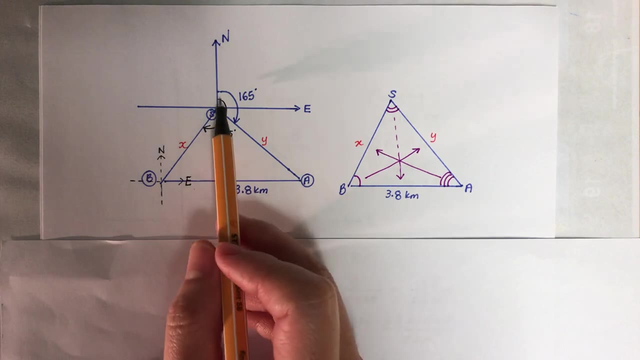 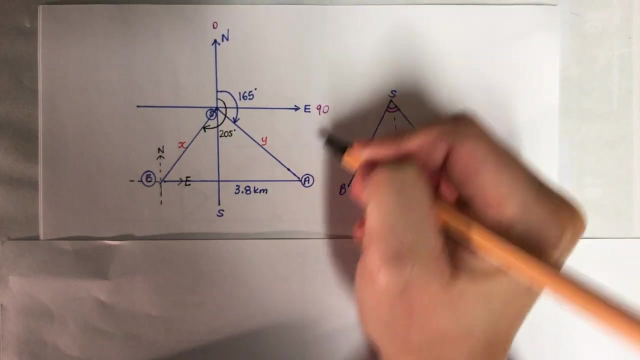 So here it is, I've got it ready. So the A was on a bearing of 165.. It's in that. you know that's what zero degrees: 90, 180, 270.. So that's where it is. 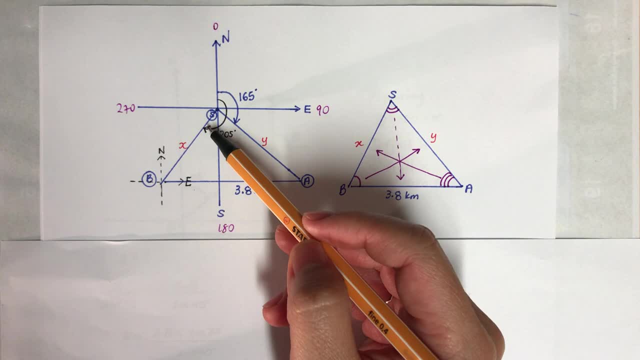 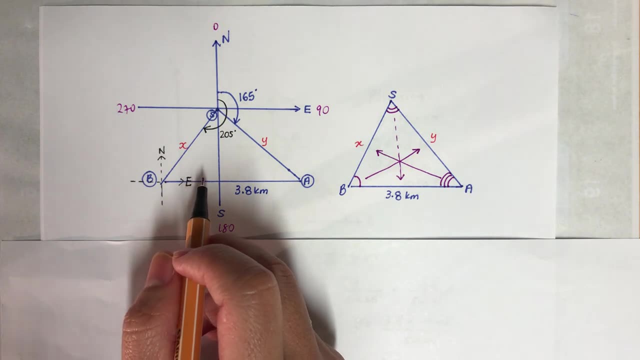 And the second one is: what Bearing of 205.. Right there, And do you remember this? It says A is due east of B, So east of B, So A is east of B. So that's if I had to draw another bearing here, starting with B. 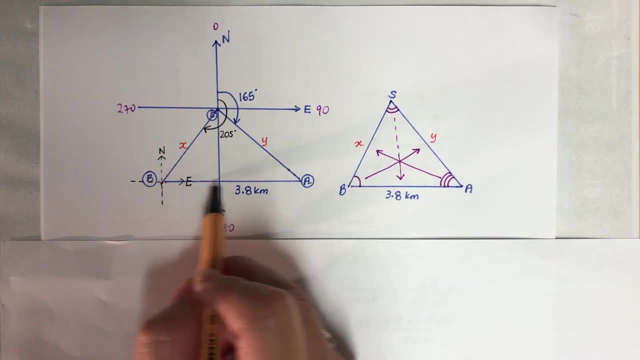 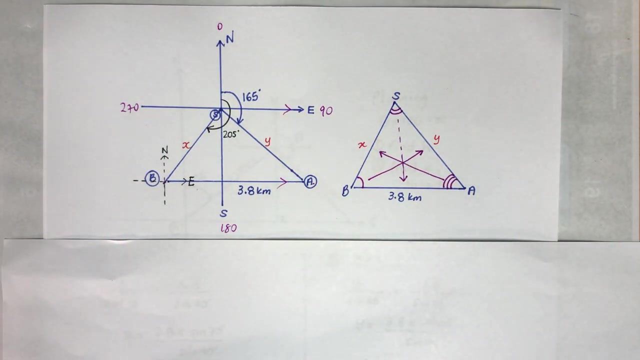 it's due east, So A is. so what does that really mean? It's this line and that is perpendicular. I mean parallel, Okay, Parallel to each other, So that's a straight line there. Okay, That's what it means by A due east of B. 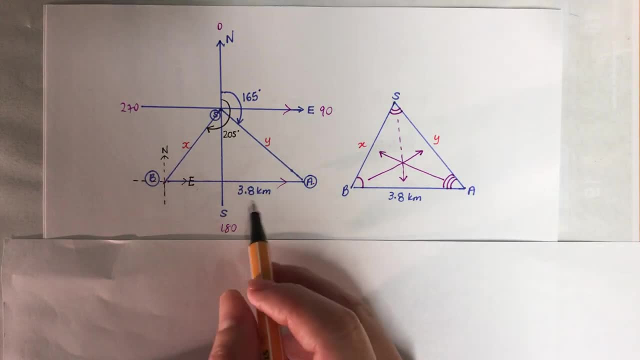 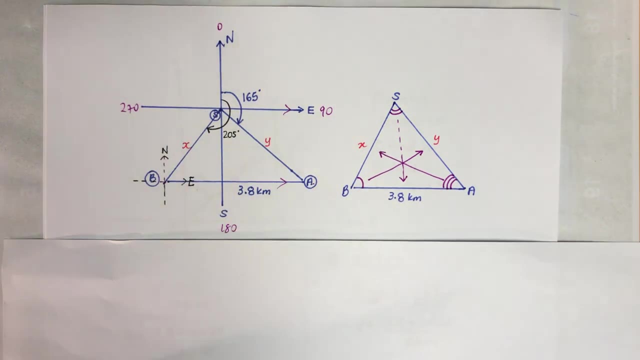 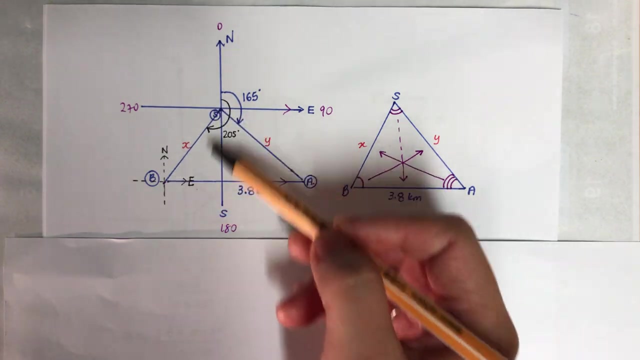 So we got. the distance between A and B is 3.8.. I've got everything I need. I've just labelled this line and that as X and Y So I can see the distance from submarine to each boats there, A and B. 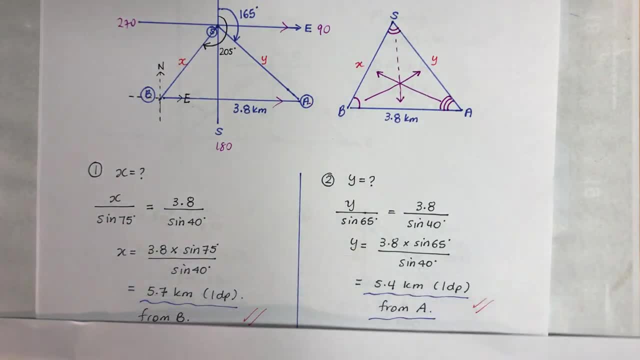 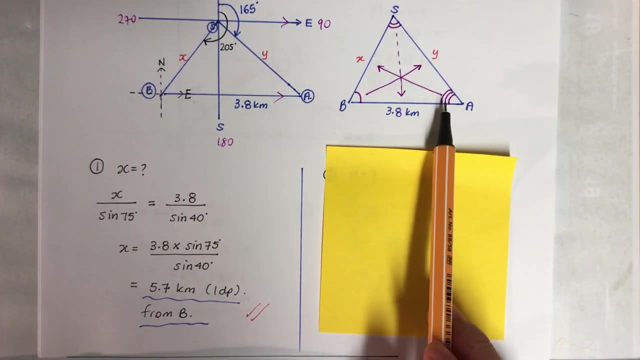 Okay, So to find, let me just cover this one, So I'll do one at a time. So X to find X, I need to find this angle and then matching up with X and this angle and that. So let's find the angle here. 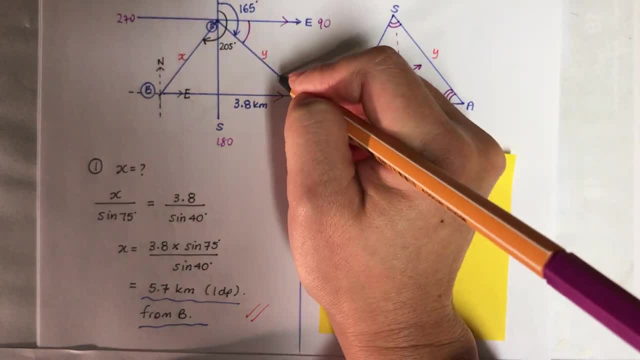 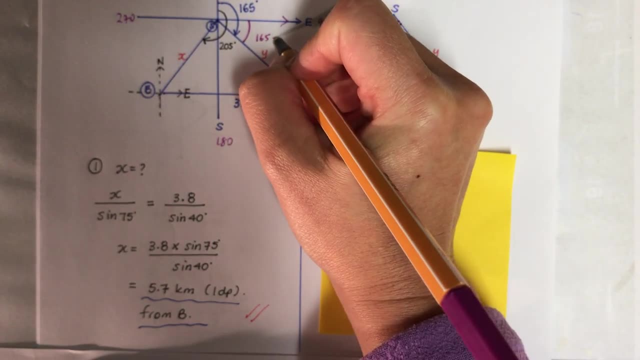 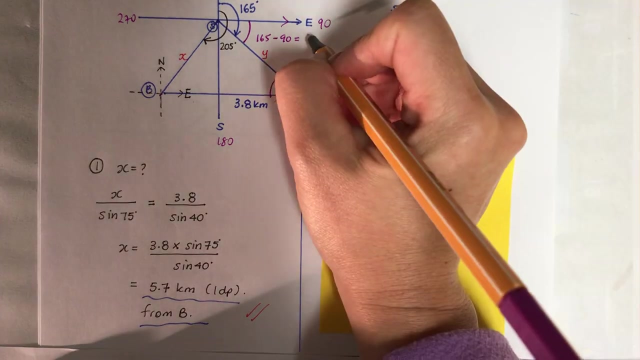 So how are we going to find this? This will be same as this, won't it? So what's this going to be? It'll be 165 take away 90.. Yeah, 165 take away 90, which is 75, which this will be 75. 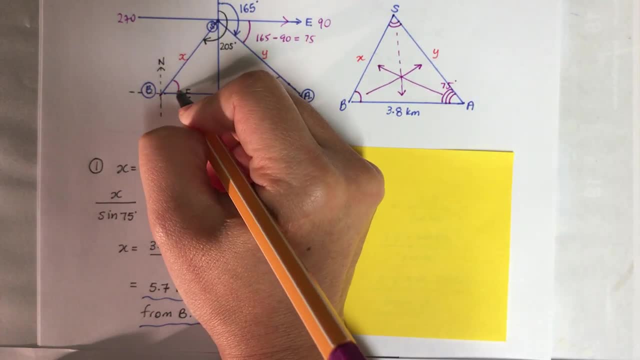 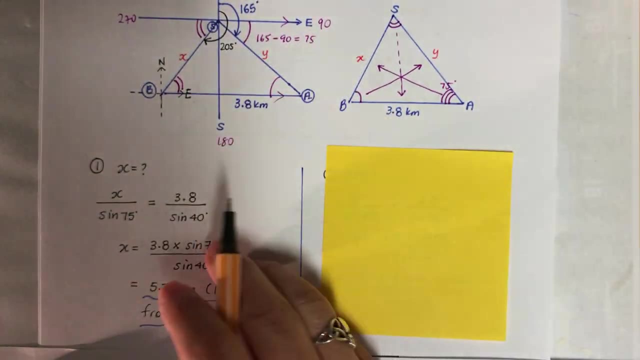 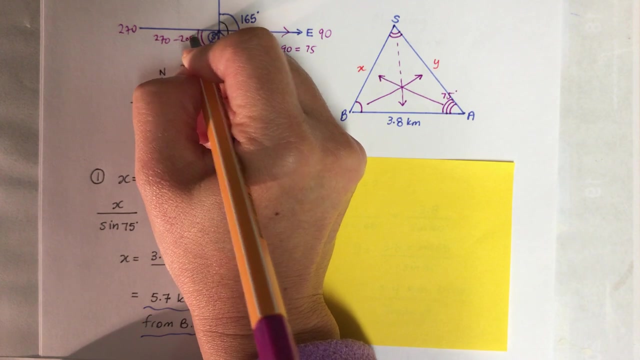 And then I'm going to find this angle by using this one. That will be same right. So how do I find that one 270, take away 205, will give me 65. So that's 65, 65.. 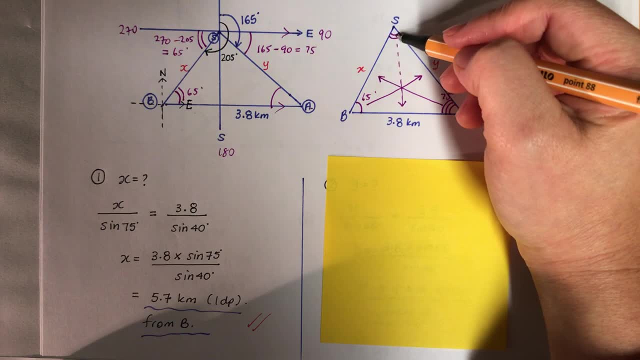 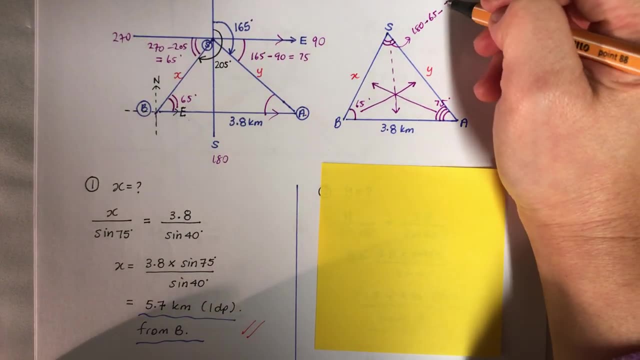 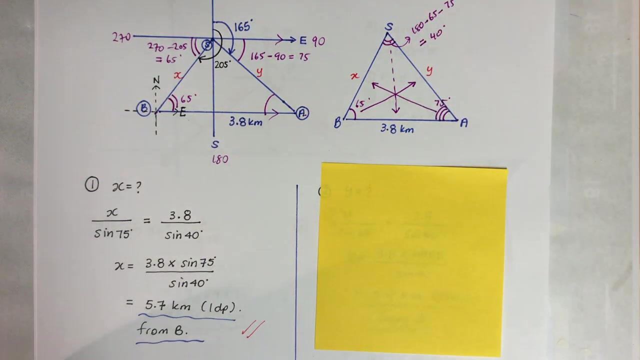 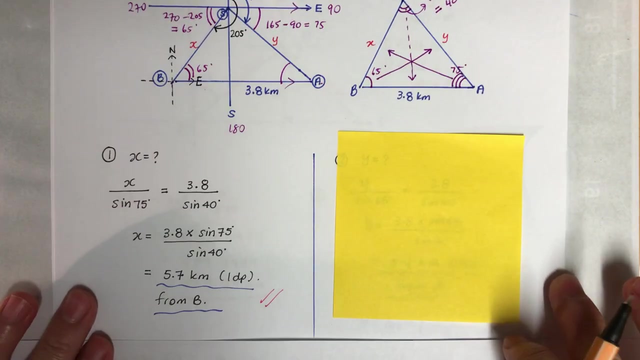 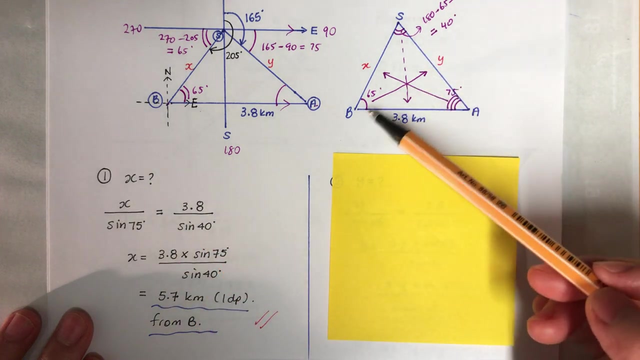 Okay, And this one, that's not bad: 180 take away 65, take away 75 will give me 40.. Isn't that? Yep? So got that. Now I can do sign rule. So X over sign 75, and 3.8 over sign 40, and I will get 5.7 kilometres from B because 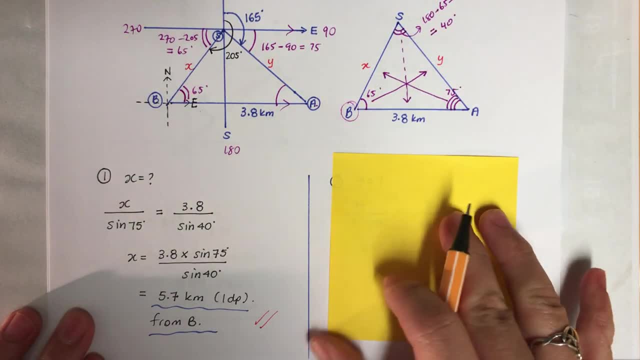 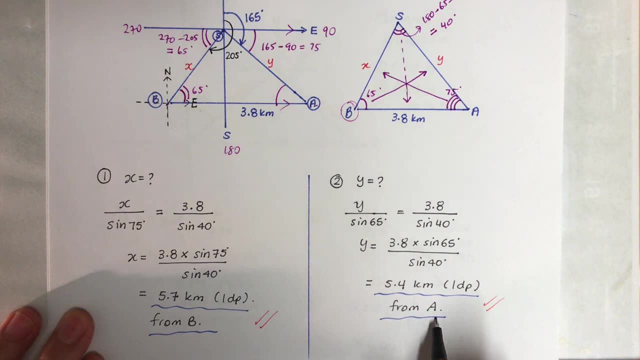 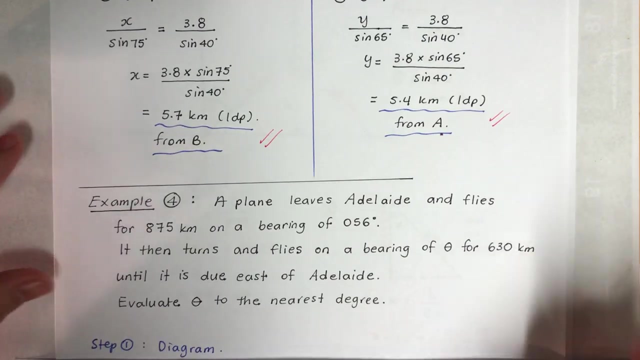 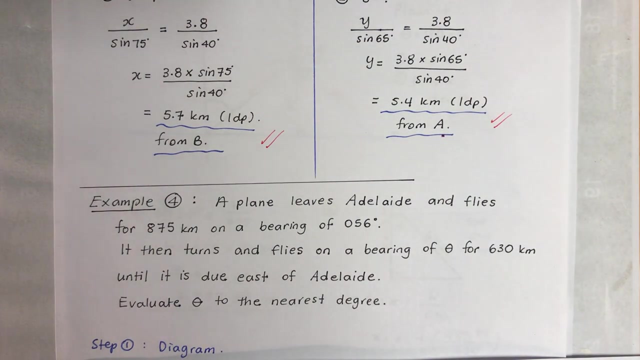 X is from B, Okay, And then the Y part: same, exactly same, but you make sure you mention from A, Okay. So that's not too bad. So example four: A plane leaves Adelaide and flies for 875 kilometres on a bearing of 56 degrees. 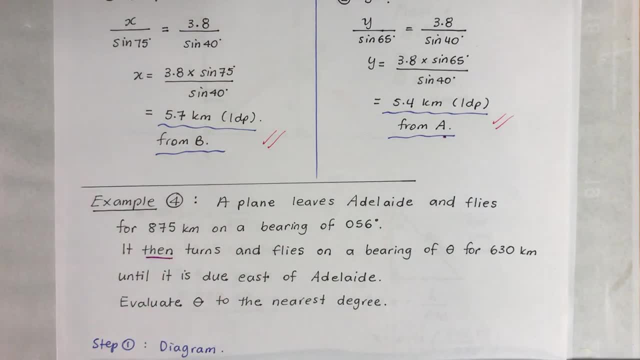 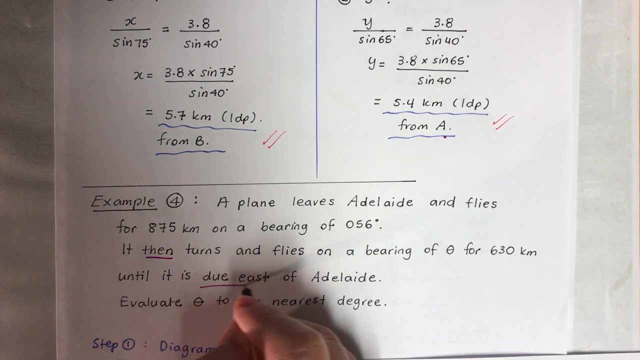 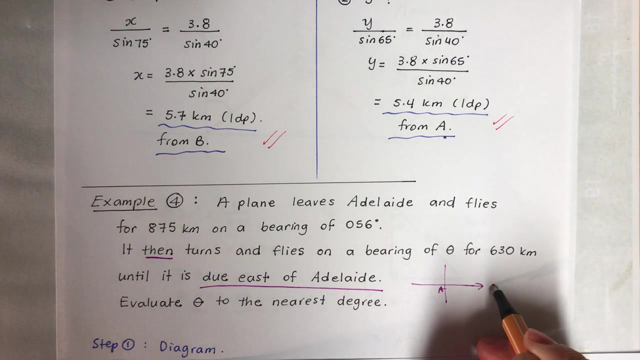 It then turns- So that's just indicating of- So turns and flies on a bearing of theta for 630 kilometres until it is due east of Adelaide. So it's on the Adelaide side east somewhere right there, Okay. 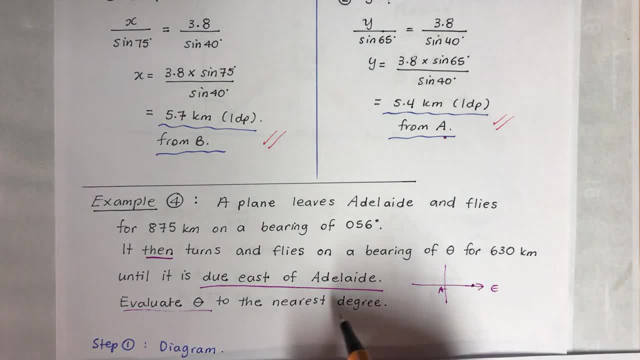 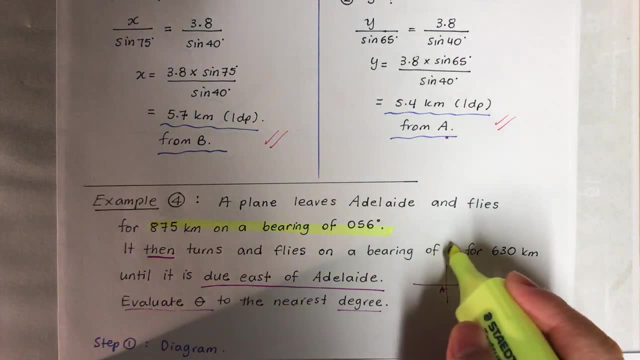 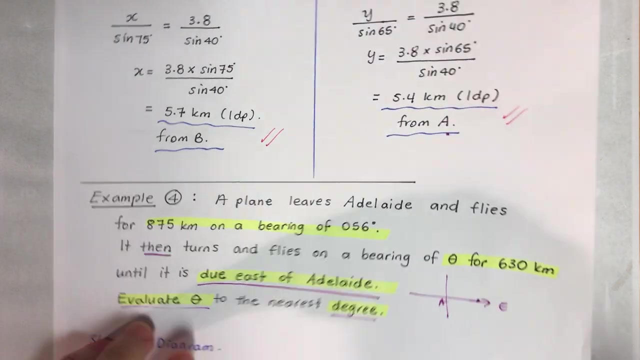 Evaluate, Find theta to the nearest degree, Okay, So, if I sort of highlight all of that, I sort of highlight all of this, Okay. So diagram is important, as I've told you before many, many times. So first thing you have to think about is the diagram. 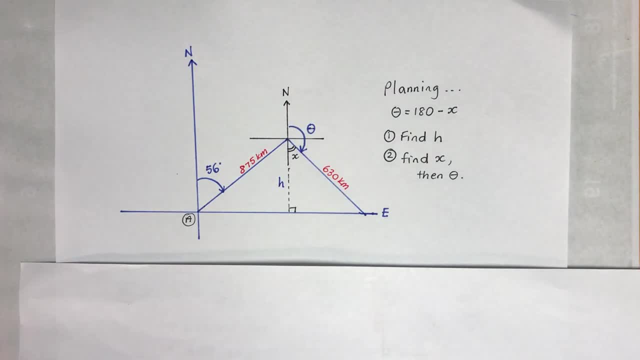 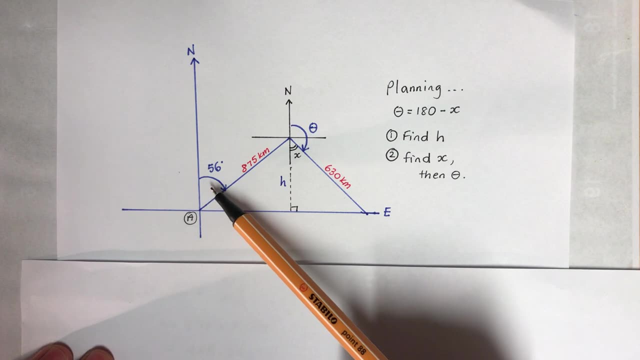 So let's have a look at this. So what happens here right now is So 56 degrees at length. Okay, So that's my Adelaide, the starting point. So plane leaves there, and it was at first 56 bearing and 875 kilometres. 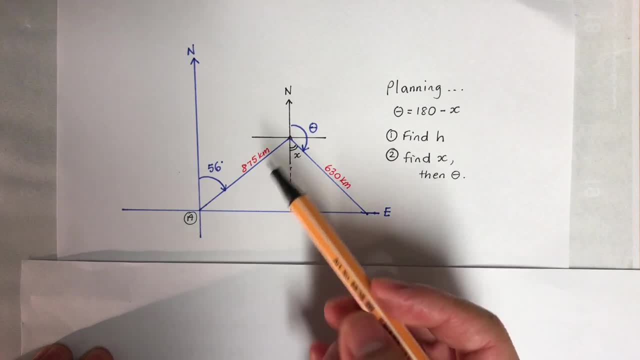 And then it turned right, Turns and then flies away. So we don't know what the bearing was, but it's going and it stops right there, due east of Adelaide, Because that's Adelaide and that's east, So it stops right there. 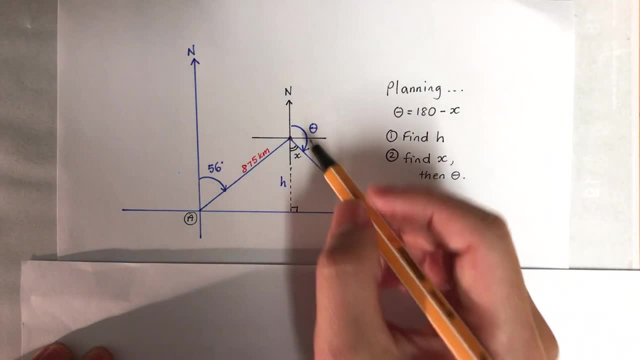 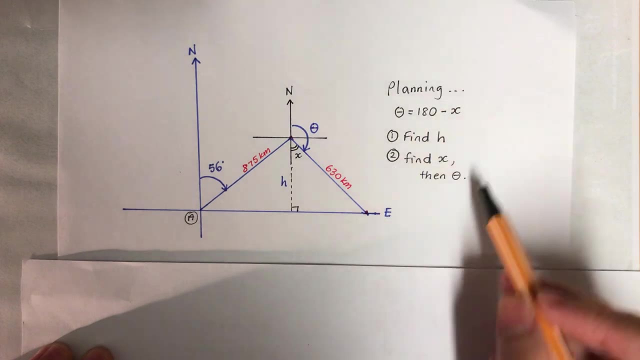 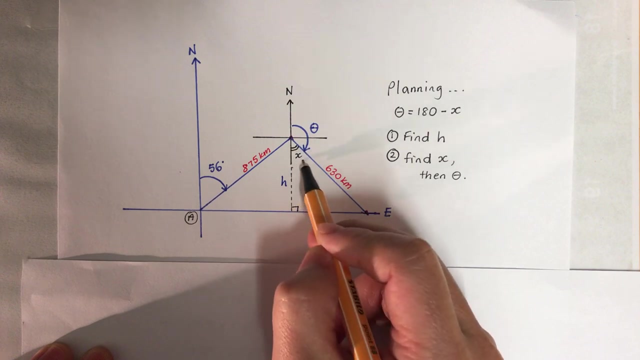 Okay, So that's what it means. Now we have to calculate the bearing. Okay, So, if I could find- So this is my plane- If I could find this little angle here, x, what I call it x. I can find bearing by taking.